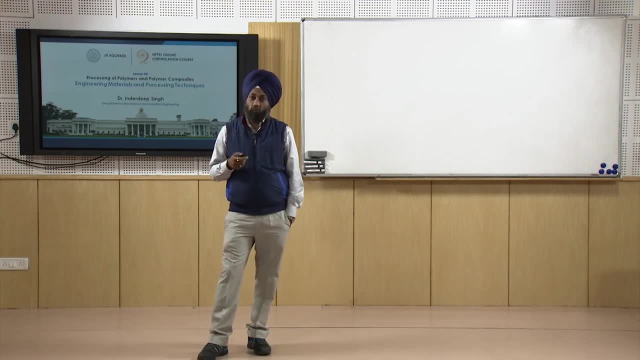 of the courses taught or the most of the manufacturing courses taught deal with metals only, and polymers and polymer composites are not a part of the UG curriculum in most of the universities. Therefore, we have planned this course in order to acquaint the learners with the fundamental aspects. 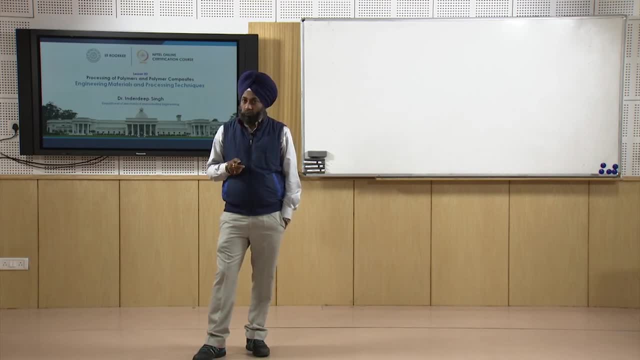 of polymers and polymer based composites, Although there are number of non-metals available, such as glasses, ceramics, and there are host of other non-metals for which the processing has to be understood by engineers and scientists, But plastics being one of the most commonly used commodity material, one of the most common 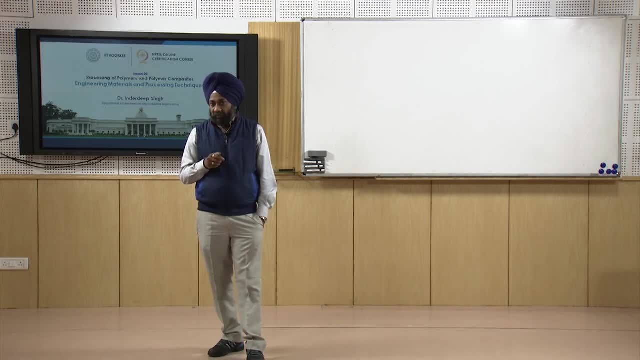 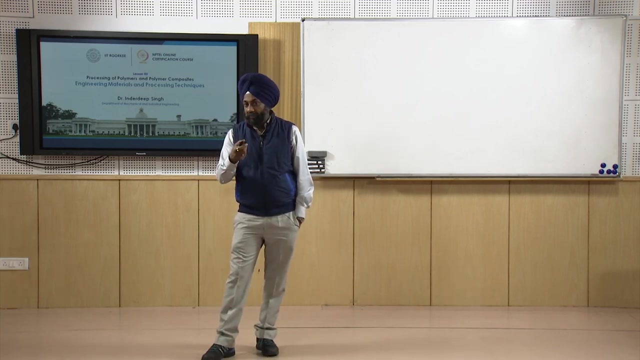 used engineering material. it was decided that we should offer some information, some fundamental information, to our under graduate students related to the processing aspect of polymers and polymer composites. I do agree that the fundamentals of polymers are taught in many universities and colleges in the course on material science, but the detailed account that how these information 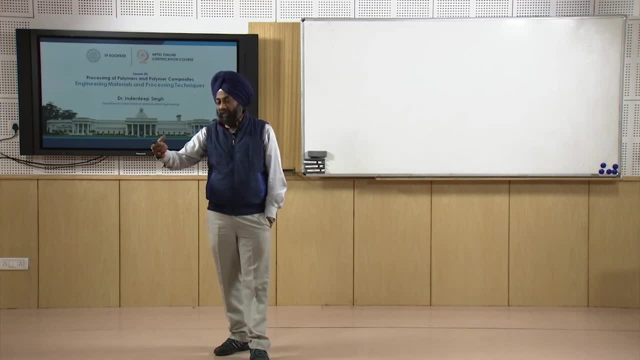 of science can be utilized, be converted into engineering, and how the products can be made is not covered in the curriculum. Therefore, we have tried to develop this course. Now we will try to understand today the two important aspects. What is the title of our course? 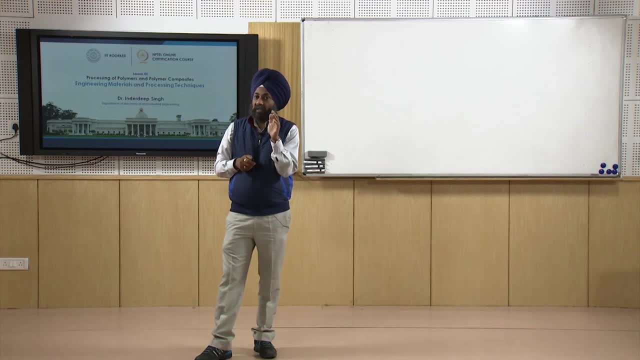 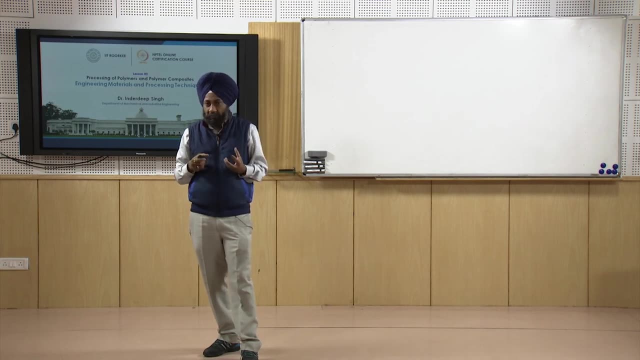 The title of our course is Processing of Polymers and Polymer Composites. So we have two materials here. maybe the basic material is same. the basic material is polymer when it is reinforced with some additives or with some. we can say fibres or 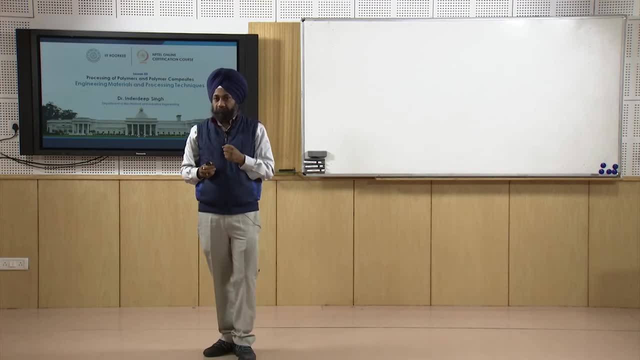 with some particles. we call it as a polymer composite. So we have a polymer and a polymer composite which we can say is a material. First part of our title is processing. So we have two things: a material and a technique, or a process and a material. 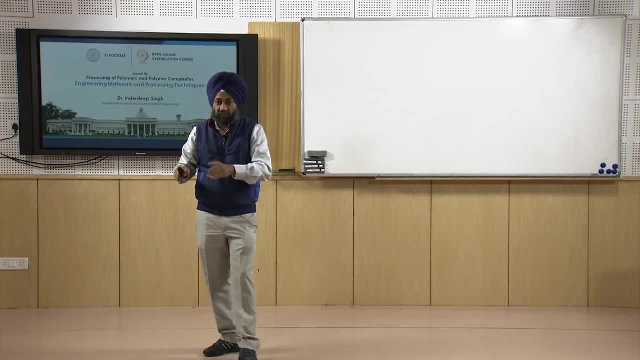 So we have to see that what are the other type of processes that are there which are used For processing of different types of materials? also, we do need to understand that this is not the only engineering material that is used in the world. there are other categories. 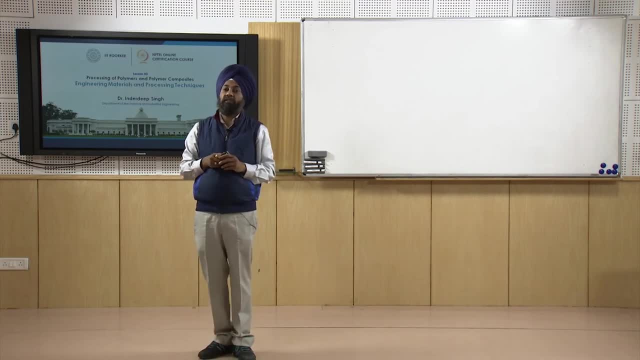 of families or other families of engineering materials that are used Now for any particular product. how to select a process- process will come later, sorry- I should say how to select a material. if you have a design in mind, you have to select. 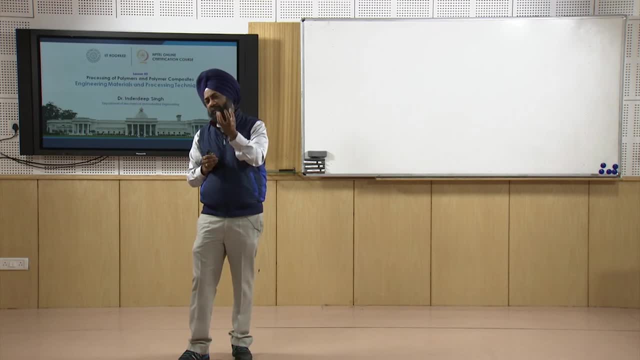 a material for that. how to select a material? what parameters come to your mind when you have to select a material? Similarly, you have decided that this product will be made by, suppose, a plastic. how to select a process? that which process is suitable for converting this plastic into its desired? 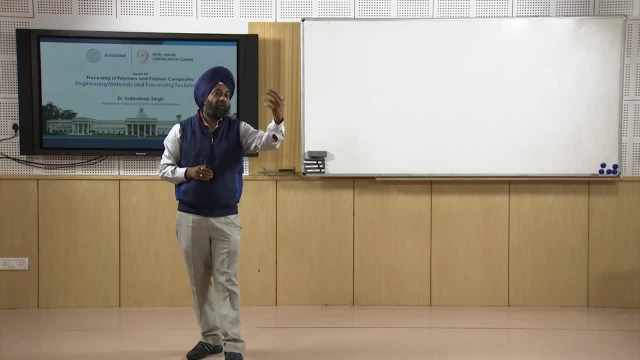 form or into the form of whatever design the designer has made. So basically there are two things: A material and a process. So we will see that what are the various engineering materials? we will also try to understand what are the various engineering processes and try to map these two things. 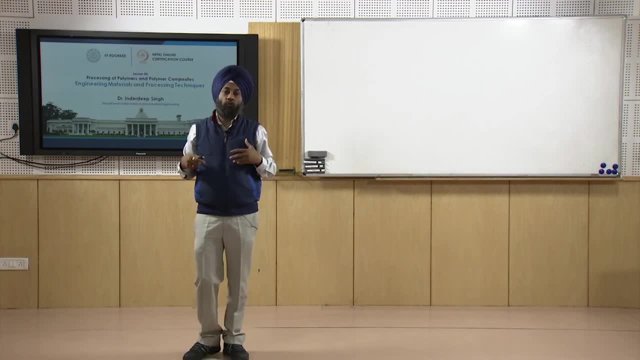 together. So for any these days, suppose I want to go and buy this jacket. what will be my target? single word that will come to my mind is the quality, that the quality of the product should be good. So if I am buying a laptop, I will say the quality of laptop should be excellent. 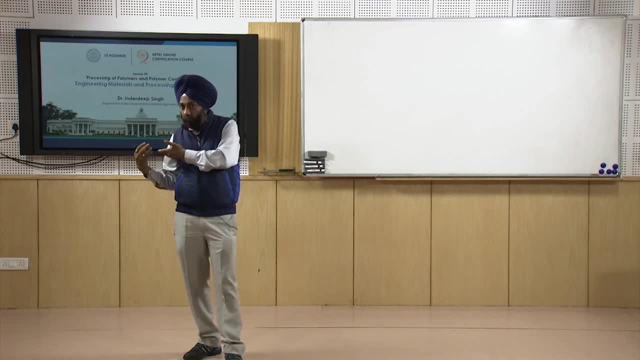 Now how quality is related to our topic. our topic is processing of polymers and polymer composites, So quality is not only related to this topic, but quality is a general perception. quality is a general thing which is related to every material, which is related to every process. 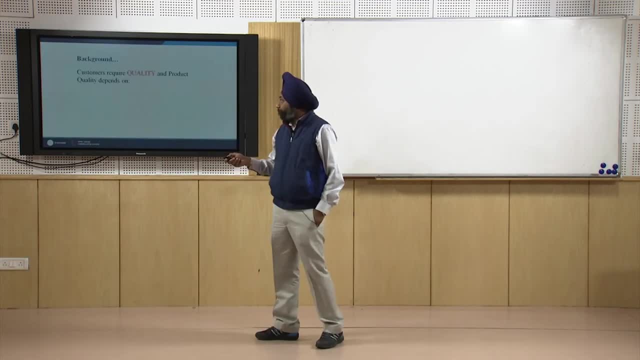 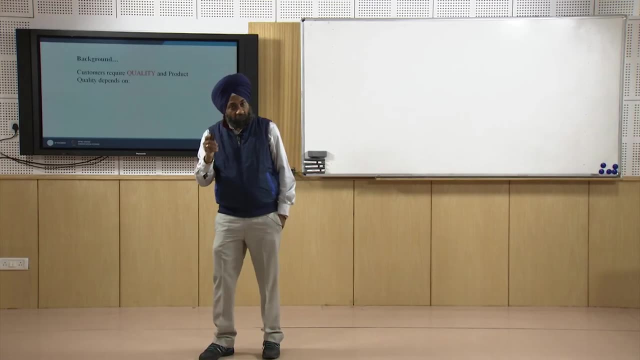 So let us see the first slide, for today, Customers require quality, and product quality depends on, starting from the fundamental thing that we should know that, why the materials are important, why the processes are important. This triangle will give you the answer to that. 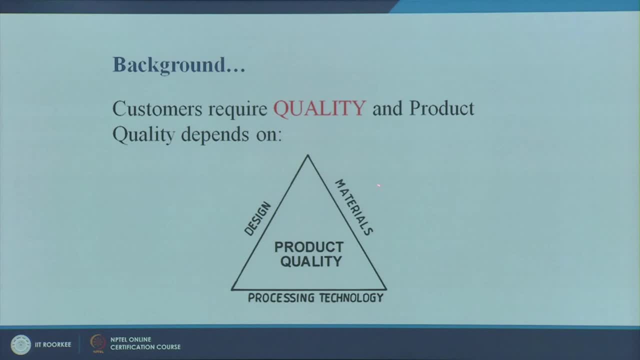 The product quality is dependent upon the materials. The product quality is also dependent upon the processing technology. 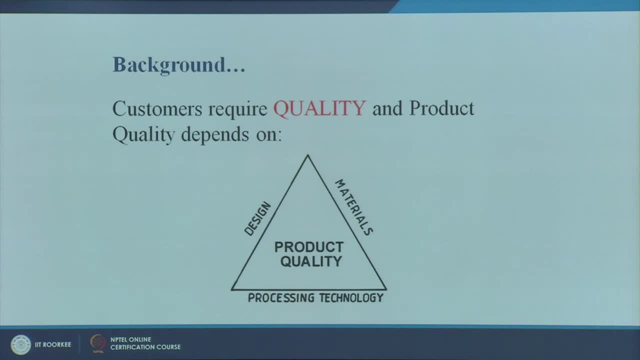 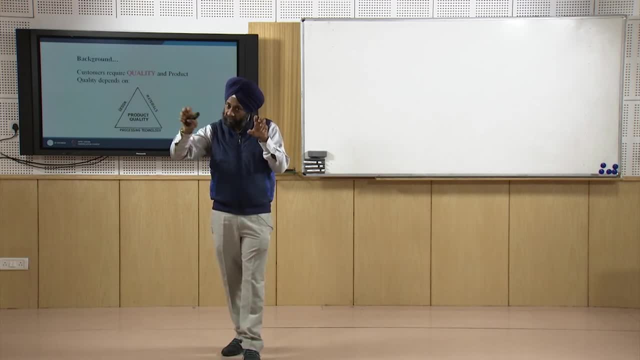 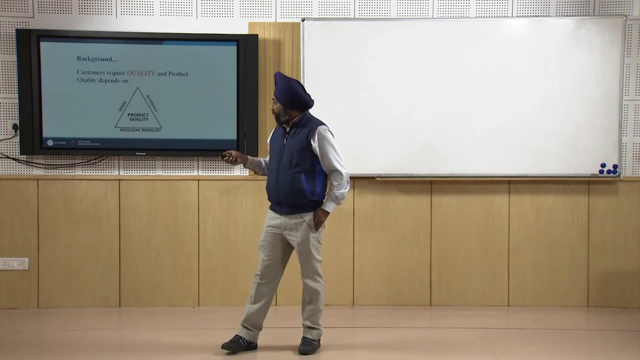 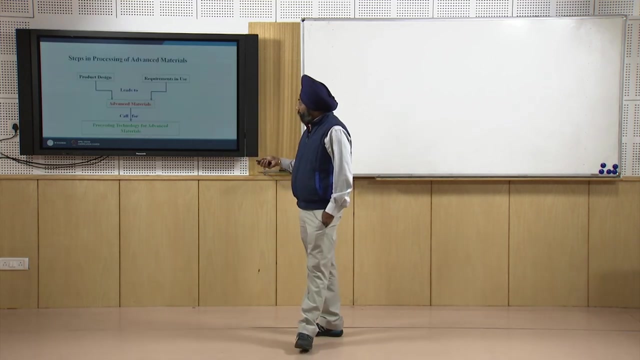 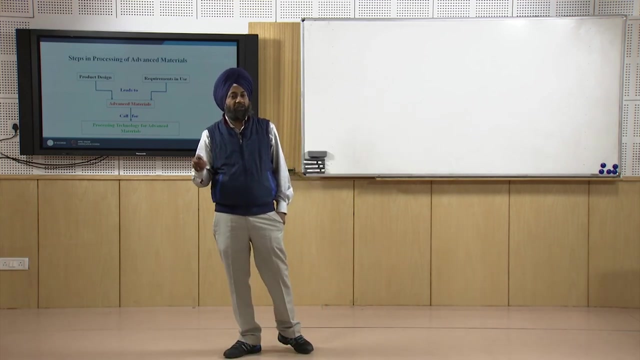 choose the appropriate material, we should choose the appropriate process, combine the two things together and then make a product which is having good quality. So materials and processing technology is very, very important to be competitive in the market. Now why there is a need for these materials, or why do we need to develop new and new materials? 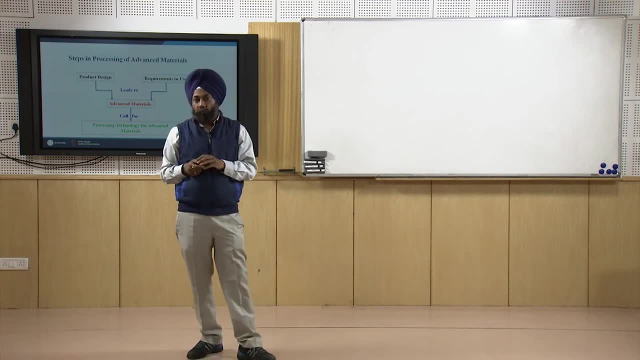 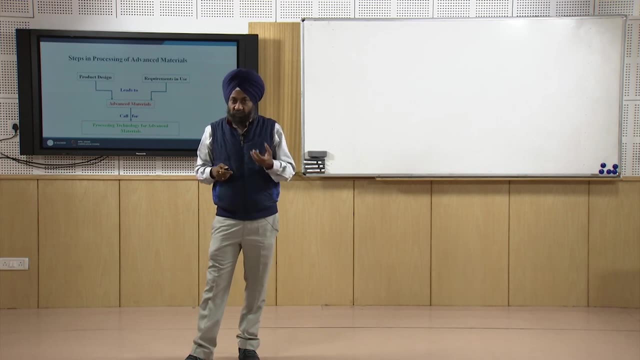 maybe somebody may be wondering that, from the historical point of view, when the metals were already known to us, what was the need of developing these non-metals? because plastics, polymers- we see most of them are synthetically processed. So what was the need when we have so many materials all around us in the universe already? 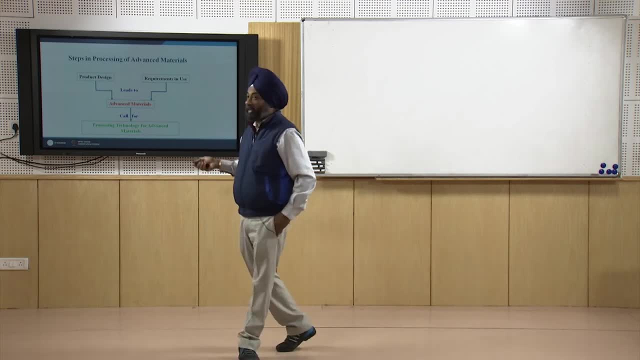 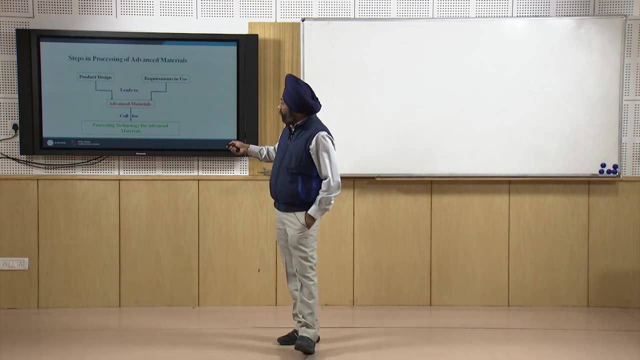 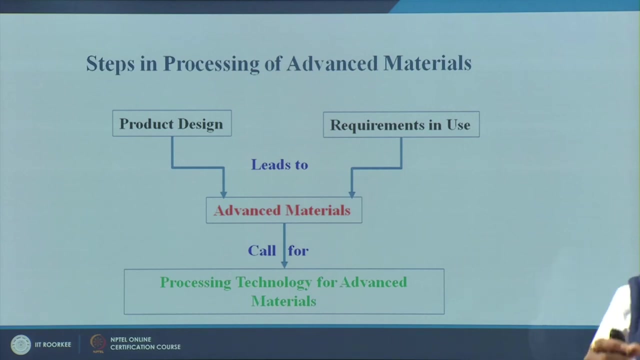 existing. what is the need of new materials? Now let us try to understand the need of materials or the need of material development. Now we see there are two terms: product design and the requirements in use. Sometimes we see the designer will design a particular product. it has to be made by. 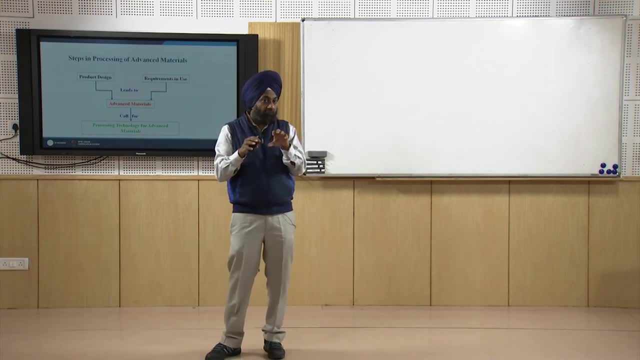 a particular material. now it is important to give that a particular shape to that material and it is not possible. maybe to give a particular shape to that specific material is not possible. then what the designer will do? the designer will have to think of an alternative material. 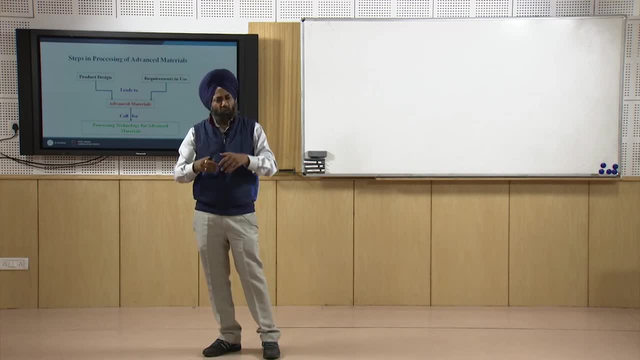 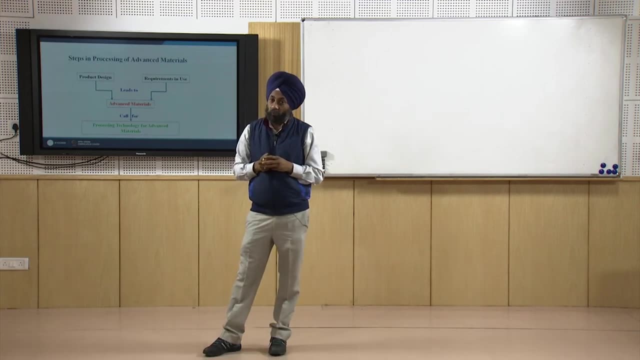 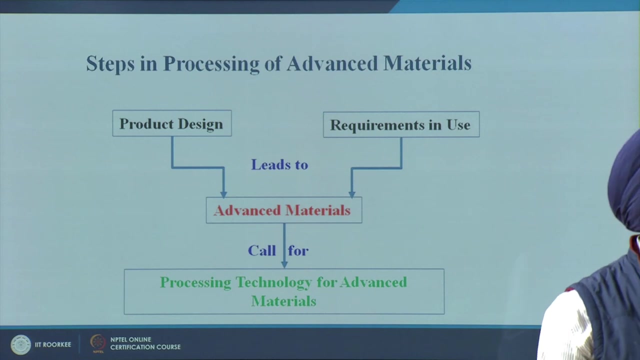 and therefore more the choice with the designer, more will be his flexibility and more will be the better or excellent will be the design that he will make out. Therefore, sometimes the product design will lead to the development of new materials because the existing materials are not able to satisfy the requirements of the designer. 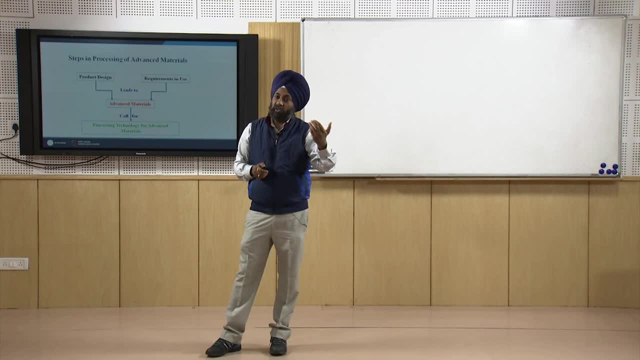 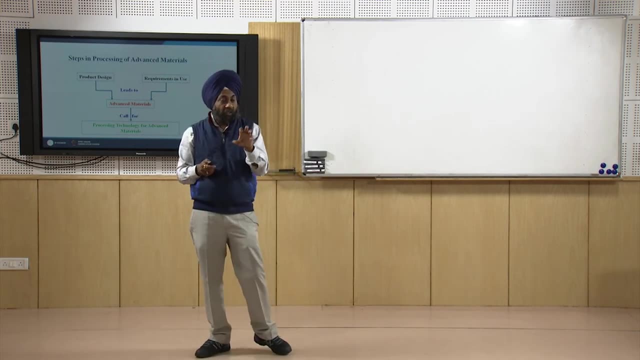 Therefore, he will have to develop, invent or find out a new material for his design, Many a times the requirements in use. for example, there is a material which has to be used for underwater applications. it cannot be a metallic because there are chances of corrosion. 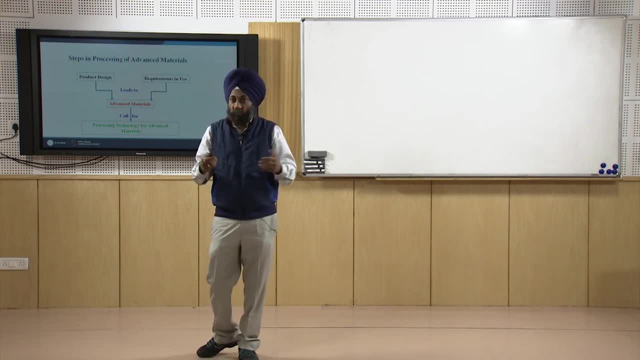 Now the designer or the maintenance professional or the engineer has to find out that what should be the material that has to be used for underwater applications. Now, this is the in service requirement: the product is under water and it has to remain there throughout its survival. 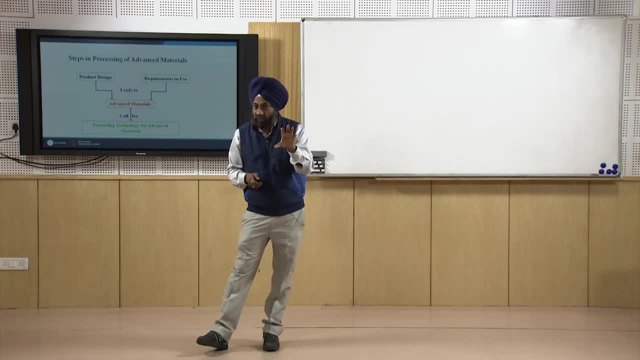 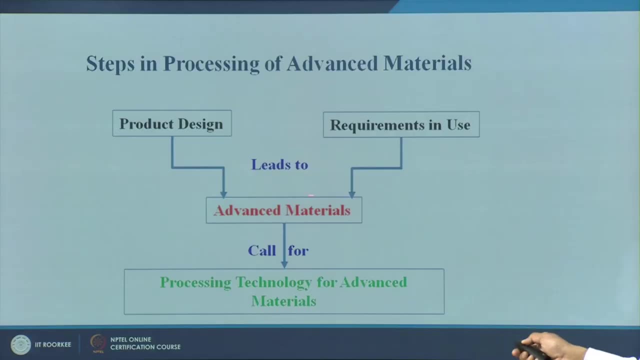 its service life. So the specific in service requirement will force the designers or force the engineers to come up with new materials. that is kind of a advanced material. So the product design and the in service requirements lead to the development of new materials. and once you have developed these new materials, for example polymers, when they may have been- 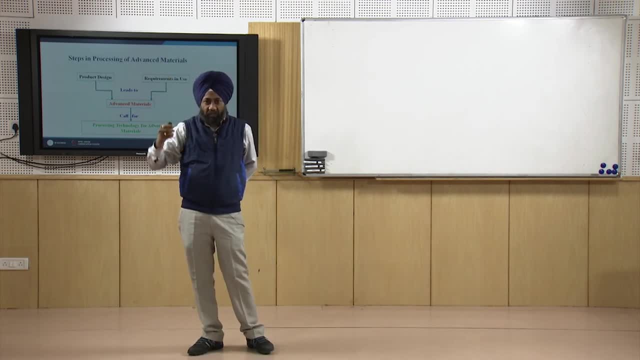 developed may be so many years back, so many decades back then. once you have a polymer, it is now the duty of the engineers, or it is the responsibility of the engineers- to convert that material into a tangible product. How to convert that material into a tangible product? you can say that is a innovation, or 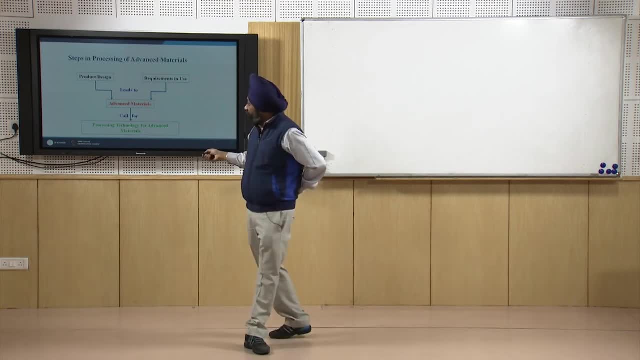 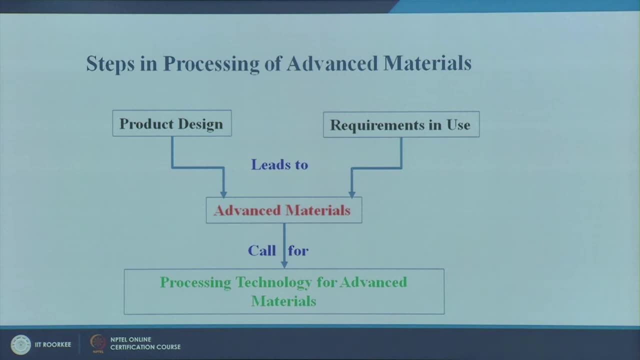 a creativity on part of an engineer. So finally, once you develop a new material, you have to find out or it will co-create all for the processing technology for that material. Similarly, when the polymers were invented, may be the next stage was to find out or develop. 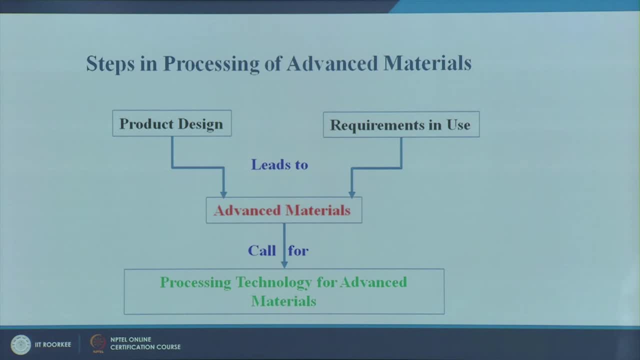 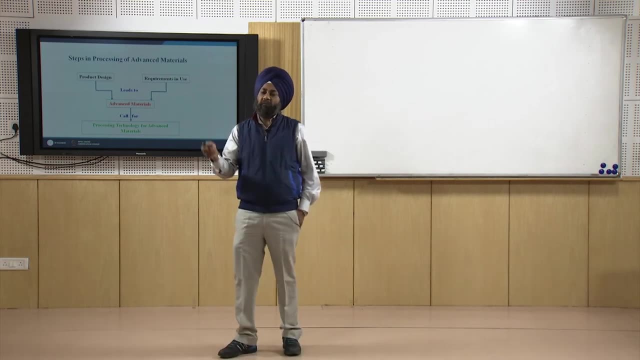 the techniques that can convert these polymers into the engineering products. So that is the fundamental aspect of coming up with new and new materials. Every day you will see there is a new material that is being developed for some certain or some specific application areas. 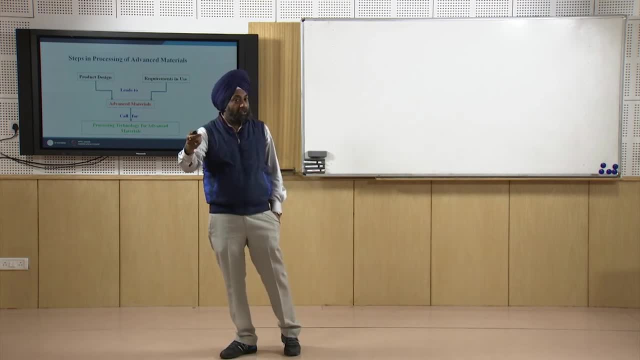 And once these materials are developed, Next stage is the development of technology, the development of techniques for processing that material in a cost effective and high quality manner, Because there may be five techniques that can be used for processing that material into a tangible product, but you will choose the technique or the technique which will be cost. 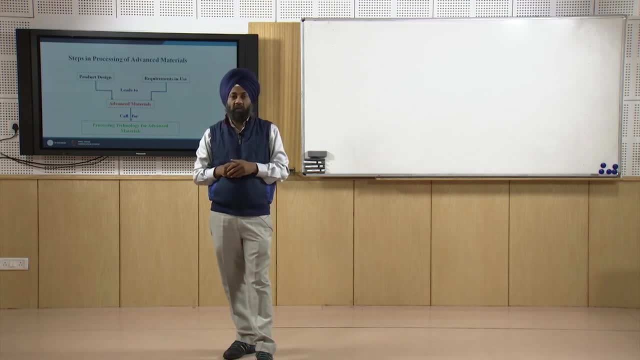 effective as well as will produce the high quality output. So there can be so many techniques, there can be so many materials. So the life of engineering Is very, very challenging: that which material should be chosen for which particular product, and how that material will be processed. which process has to be chosen for that material. 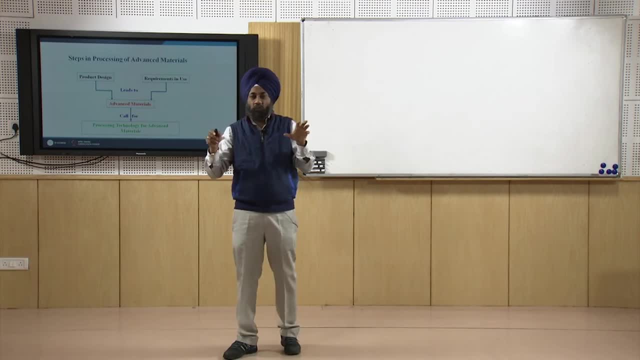 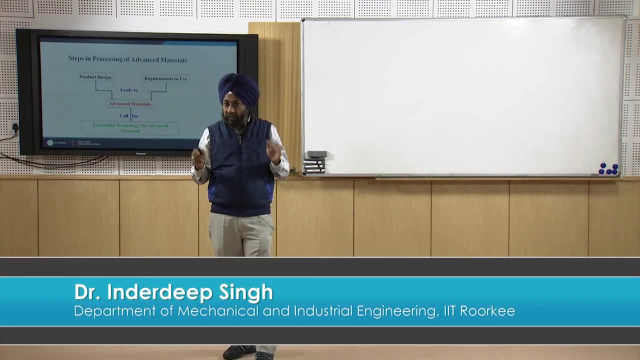 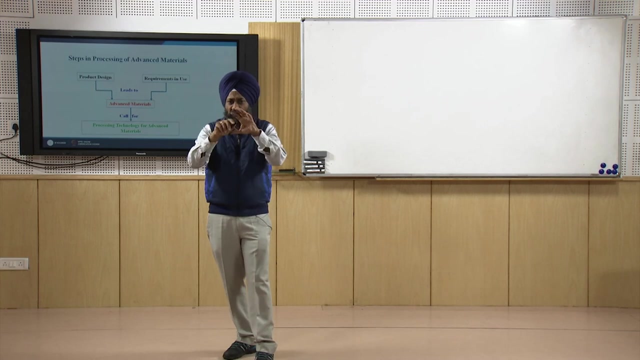 in order to convert it into a product. So we will try to understand. we may not be able to address everything in detail, but we will be able to at least highlight that what are the various engineering materials, What are the various manufacturing processes And how they club with each other. 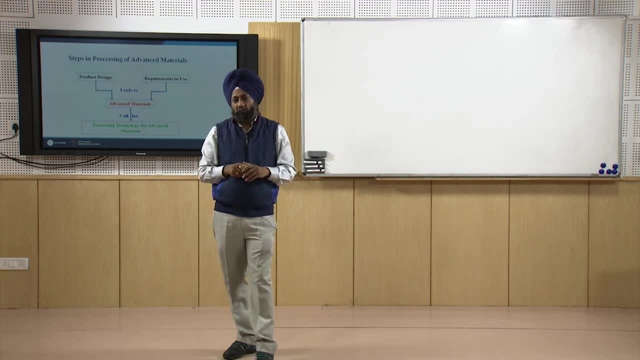 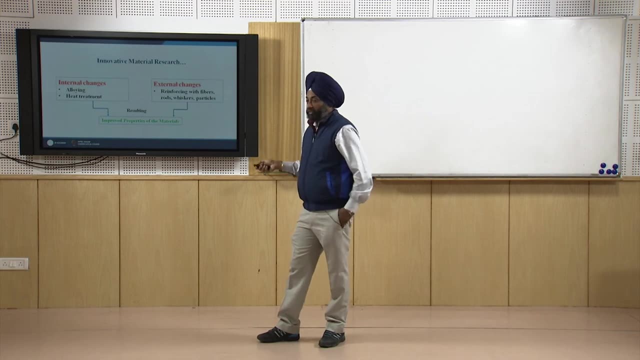 So that is the first stage. Which other, which process is suitable for which particular material? that we will try to understand Now how, once you know that there is a requirement for coming up with a new material, usually we see we make some internal changes in the material. for example, for metals we may have. 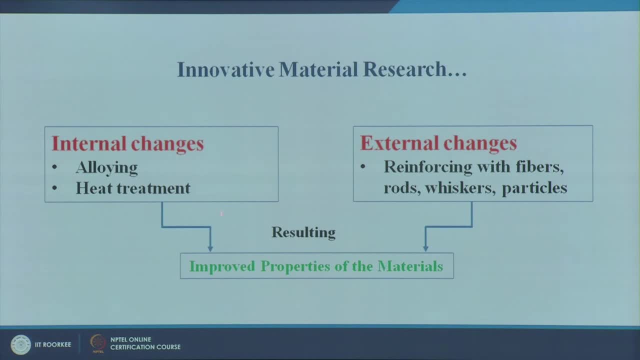 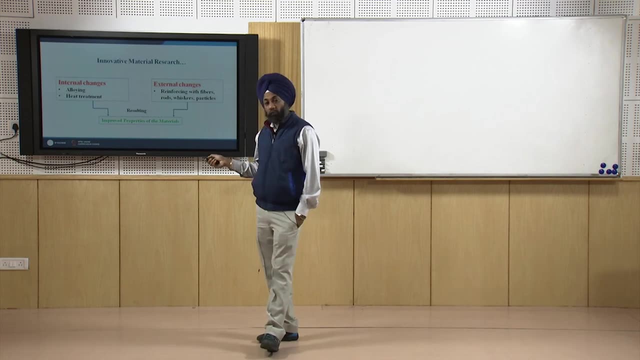 we may develop alloys of that metal. we can do heat treatment to force some micro structural changes in the metals In order to give them the specific properties, because we have to come up with a new material which is going to satisfy our specific requirement. or we can do some external changes. we can. 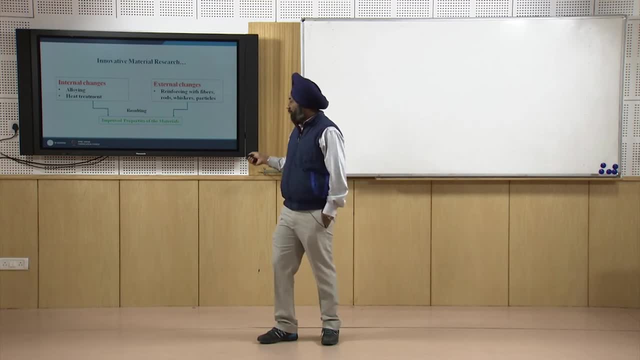 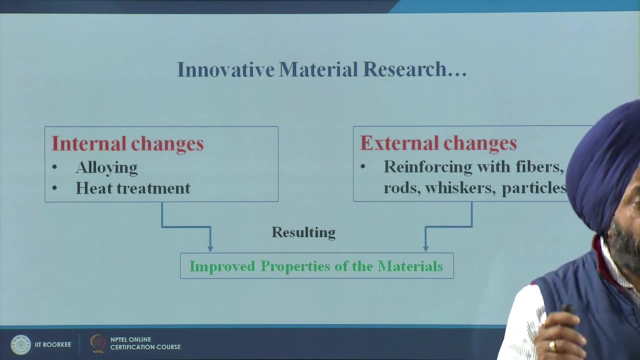 add some fibres, rods, whiskers or particles into a matrix or into the base material and try to change the properties of that material. So we can do internal changes, we can do external changes and the resultant material will have the improved properties. So this slide has specifically been included in our discussion because we are going to 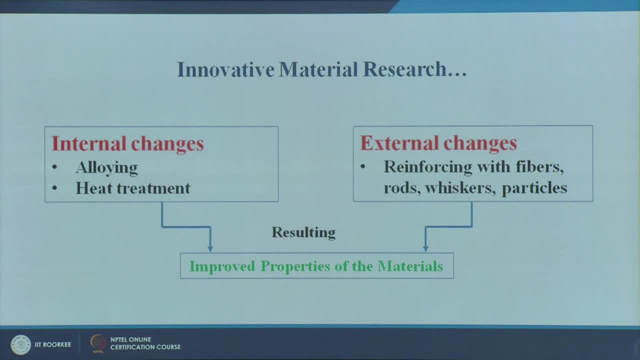 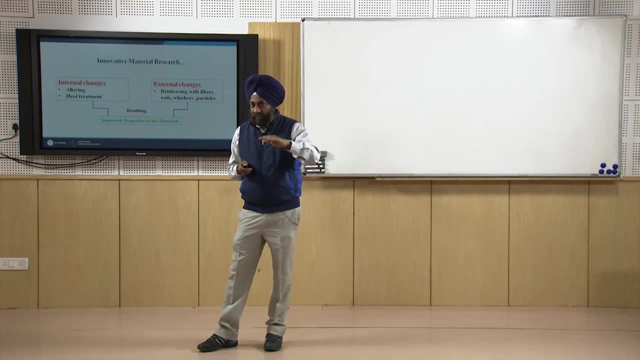 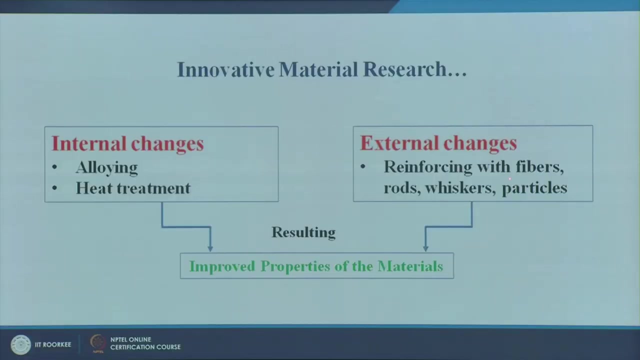 talk about the polymer based composites also, and the title of our course is processing of polymers, which are, we can say, base materials and polymer composites. So polymer composites will fall in this external changes category, where the basic polymer or plastic will be reinforced with fillers or particles in order to improve the properties. 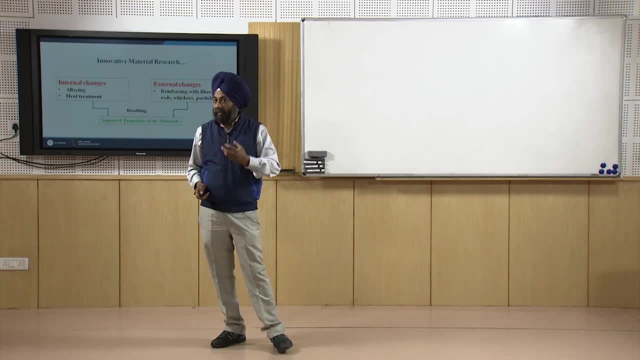 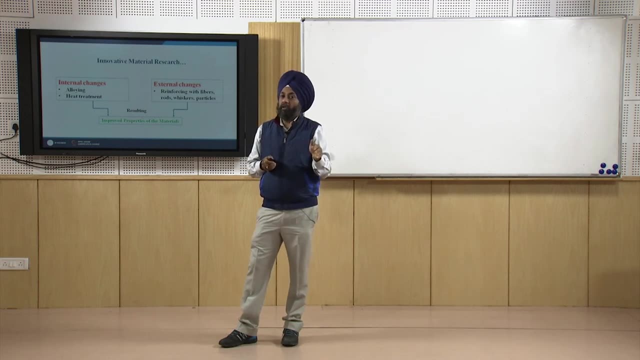 of the basic polymer or the polymer matrix, So that we will try to see there- and this slide highlights the title of our course, that is, polymers and polymer composites- because we need to change the polymers into polymer composites in order to improve their properties. 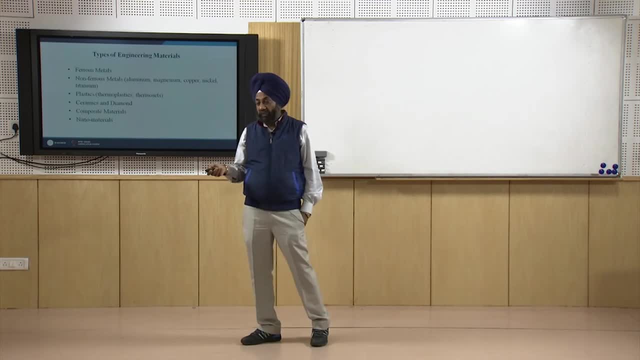 Now this slide, a very busy slide on your screen you can see. This is the types of engineering materials. this slide can be contested also. Some of the students may say no, there are number of materials which have not been included in this list, but as far as I am concerned, I feel that this summarizes may be mostly. 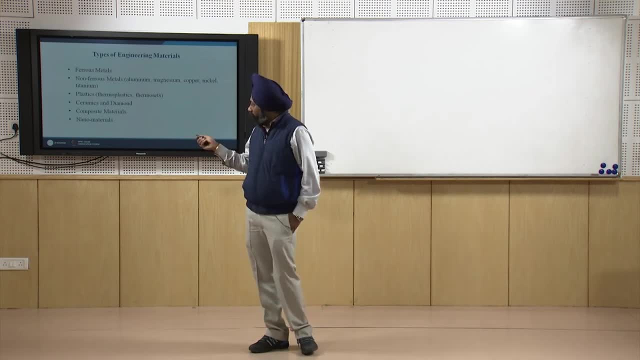 materials which we see all around us? No, but there can be no list. it is a very exhaustive, we can say, area of engineering materials, where- or I should not say engineering materials, materials- So many different, diverse types of materials exist in this universe, which is very 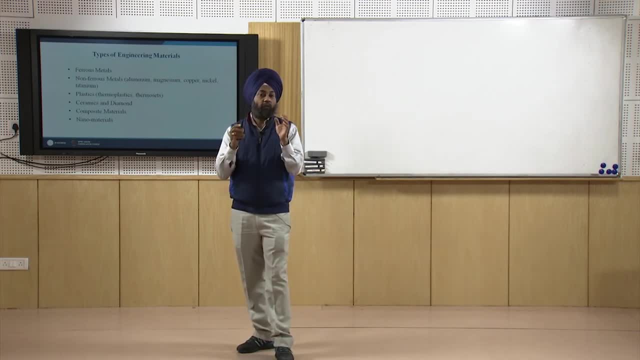 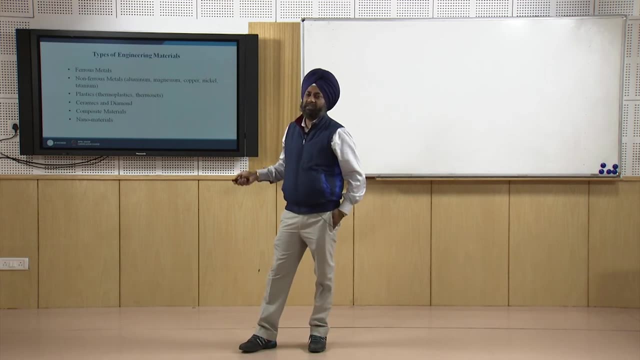 difficult to put them on one slide, But if we say engineering materials, engineering products that we see around us, we will see that this list can suffice. This list is sufficient to maybe classify the materials that we use in engineering. So let us see, maybe, if you are doing this course, 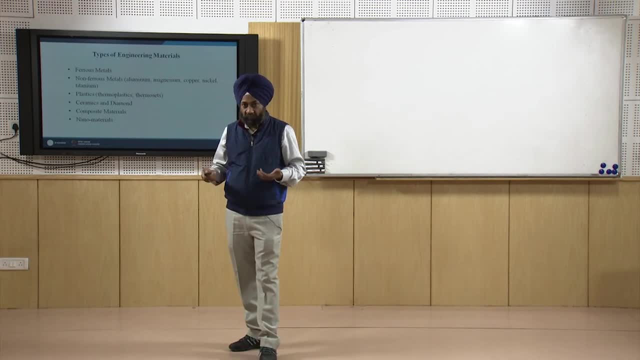 and you see this list in our this lecture 2 in week 1.. One exercise I can give you: When you are sitting in your room or classroom or bedroom, wherever you are undergoing this discussion or wherever you are listening to this discussion, you can just look around you and try to list. 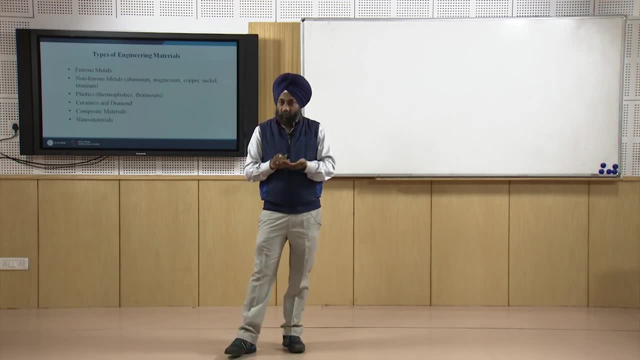 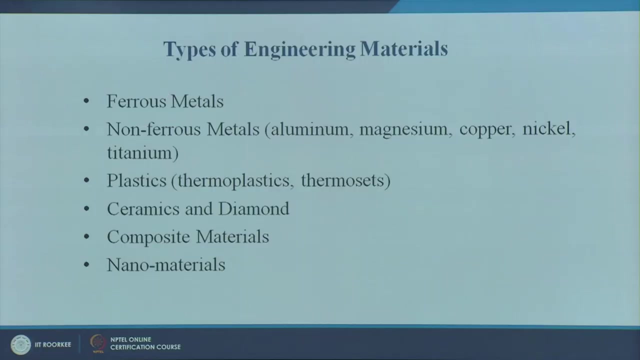 take a pen and a paper and try to list at least 5 to 7 to 10 materials and then try to fix or club them, Those materials, or map those materials or put those materials in this list. So you will see that most of the materials you will see. maybe they may be ferrous metals, They may be non-ferrous. 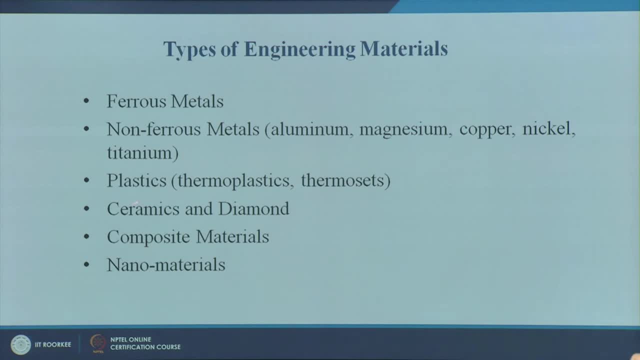 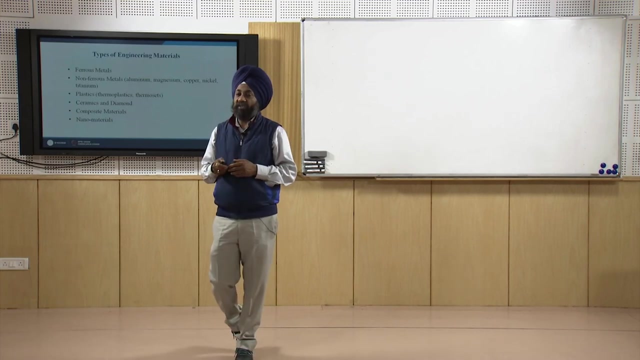 metals like aluminium, magnesium. They can be plastics- That is our course- Polymers and polymer composites. They can be ceramics or diamond Composite materials. They can be nano materials- Nano, of course. maybe we may not be able to see with naked eye. 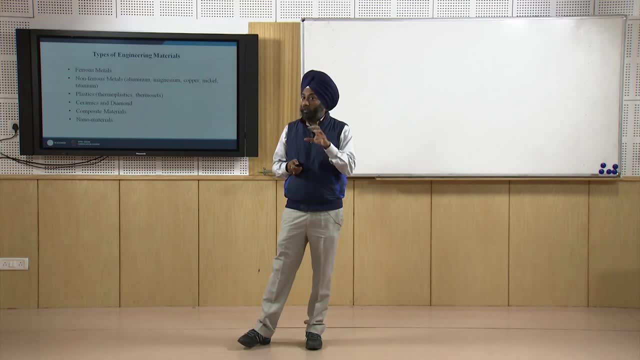 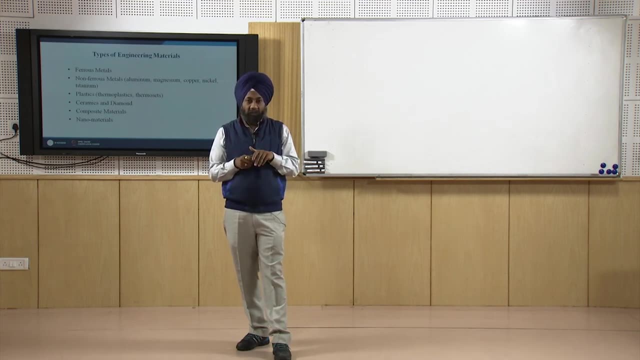 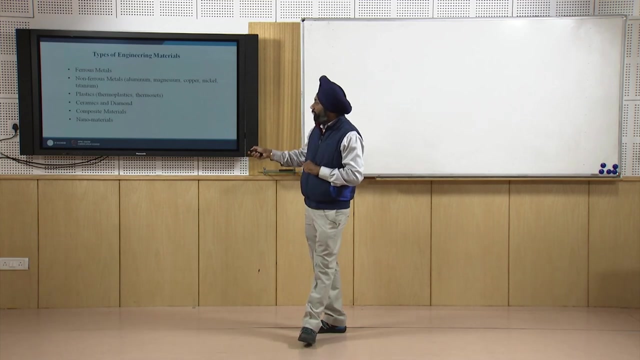 But some application of nano materials can be there. So if you do this exercise, you take a pen and a paper and you write down maybe around 10 materials that you see around you. all engineering materials must fall in any of these categories. Now, coming on to our specific or special focus. our special focus here is this number 3.. That 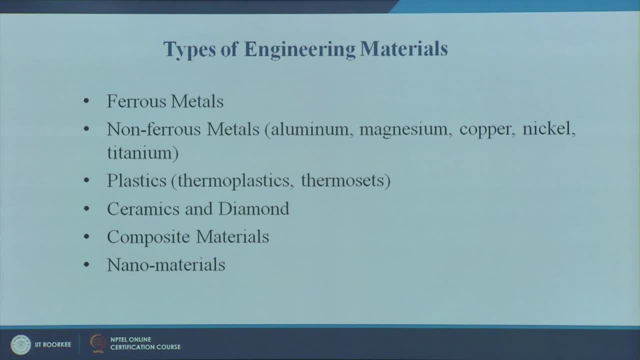 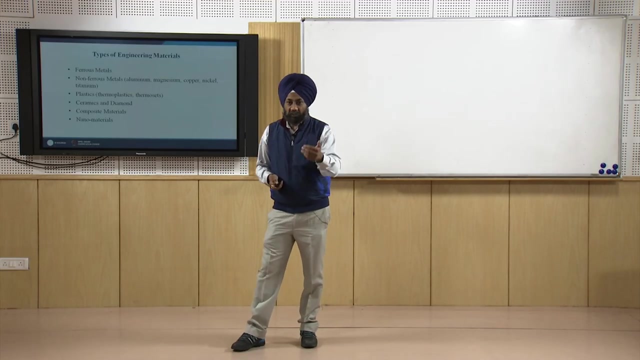 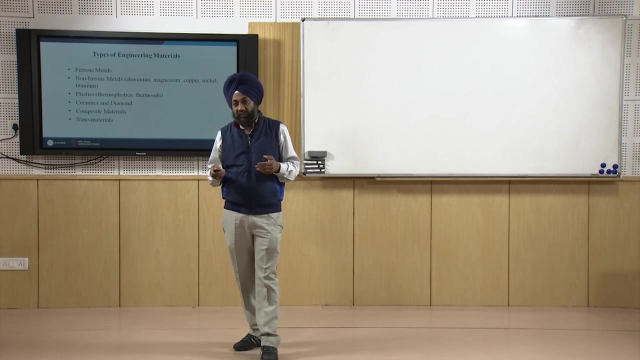 is plastics And the composite materials. So our focus is bullet number 3 and bullet number 5, that is, plastics and composite materials. Alright, as I have already highlighted, lot of discussions, lot of books are available on ferrous metals, non-ferrous metals, the processing or processing techniques or manufacturing. 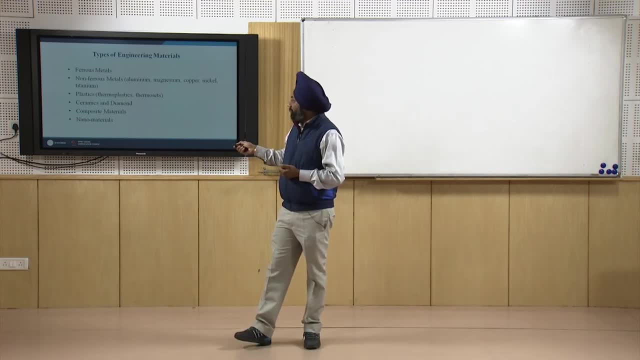 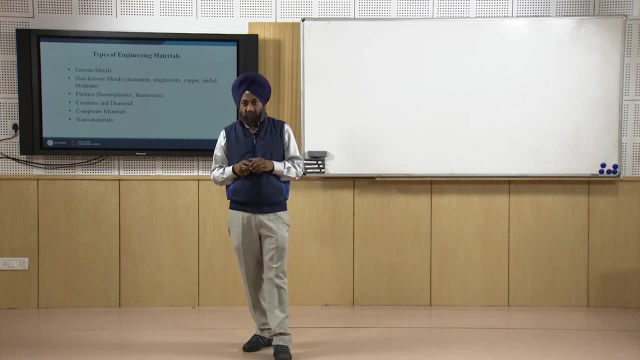 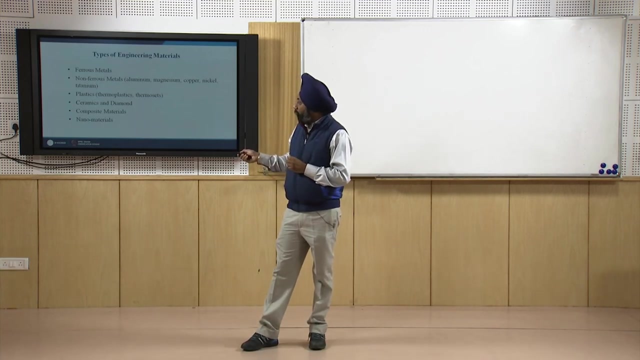 techniques or fabricating techniques for these materials- ferrous metals and non-ferrous metals- But for non-metals, such as plastics and ceramics, not much discussion is there or available for the undergraduate student. Therefore, this course has been designed So our focus would be on bullet number 3 and bullet number 5.. 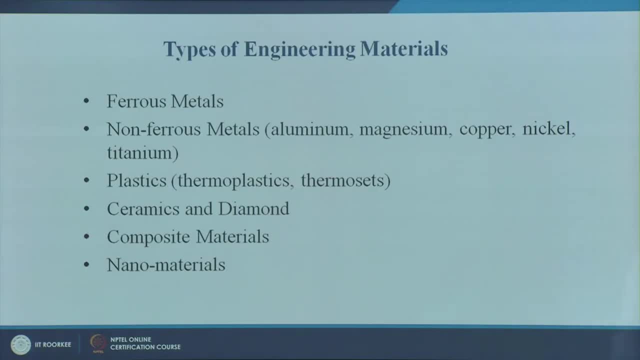 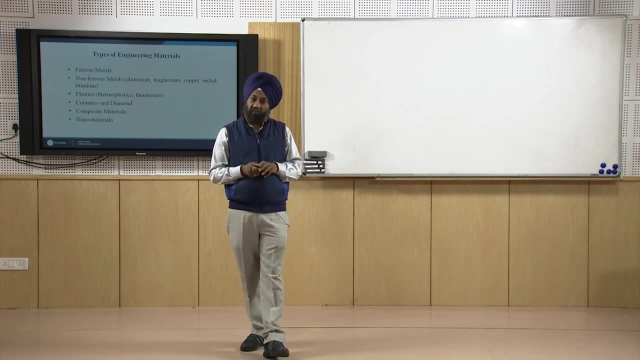 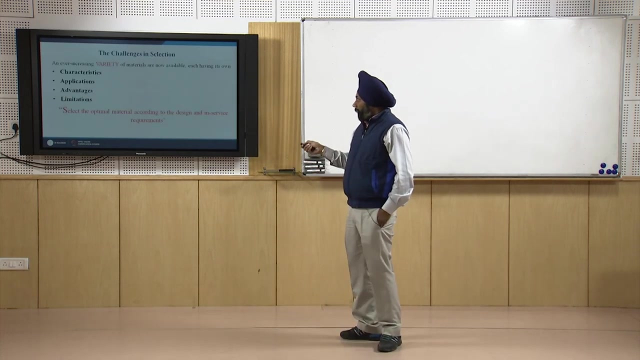 Now, these are the, this is the list, or these are the materials which are used for making engineering products. Now, what can be the processes that are used for converting these raw materials or these materials into engineering products? Let us see, We will go to that discussion. 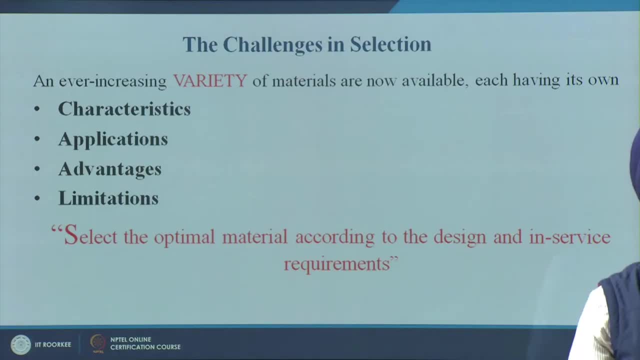 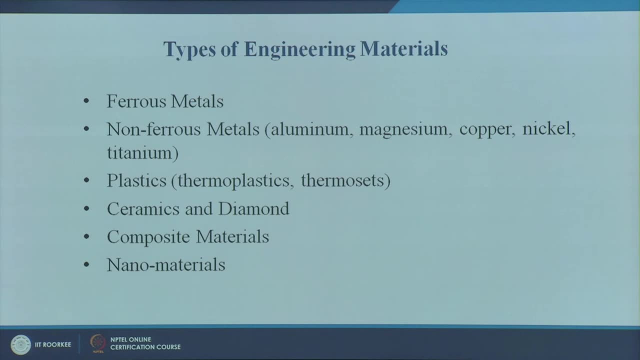 First, let us see that when you have a wide variety of engineering materials, you can see we have ferrous, non-ferrous plastics, ceramics, composites and nano materials. When we have plenty of options available with us, how to select a particular material for? 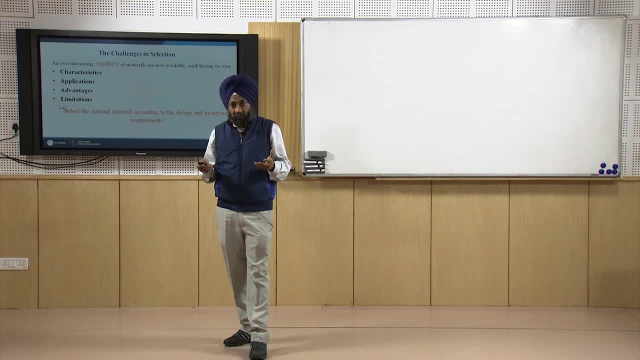 a particular application. It is a challenging thing. Same product can be made by a metal. Same product can be made by a plastic. If you have a plastic, If I ask you, give me an example- A product that is made both. it can be made by a plastic. also it can be made by a metal. 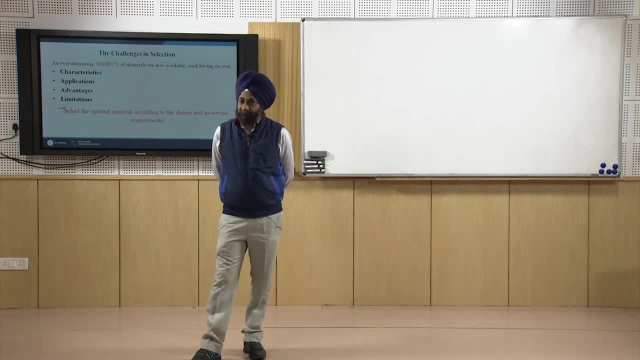 also. Just think over it. I think some of you may have got the answer to that question. If you see the chairs, You can have the plastic chairs also, You can have the metallic chairs also, And on top of that you can have a wooden chair also. 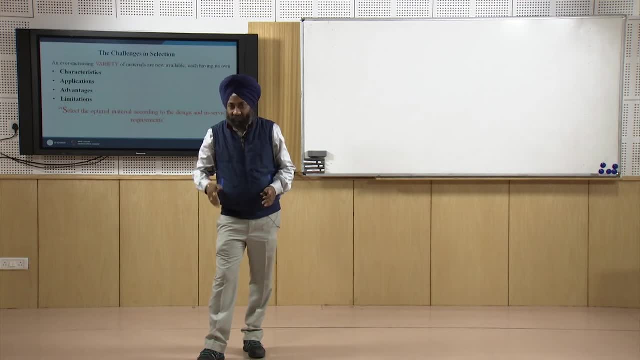 So you see that there is a list of engineering materials. Ok, There is a single product and three types of these materials can be used for satisfying the same need: that is, making a chair. So there is always a challenge of selection, that how to select appropriate material for. 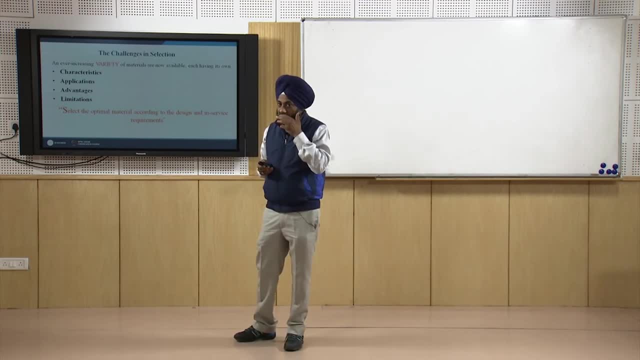 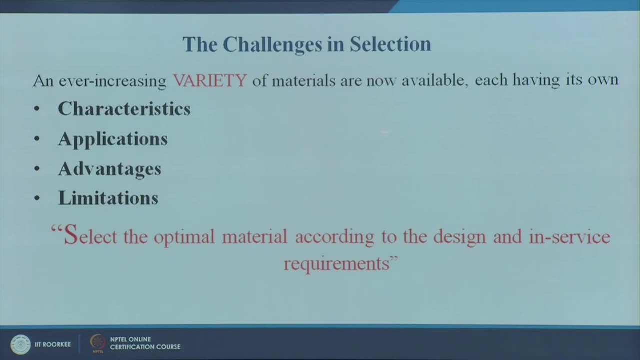 appropriate application. So you have a list of materials. So what will help you? The following things will help you. An ever increasing variety of materials are now available. The variety I have already listed in the previous slide: Metals, non-metals, polymers, ceramics, diamond, nano materials, composite materials. 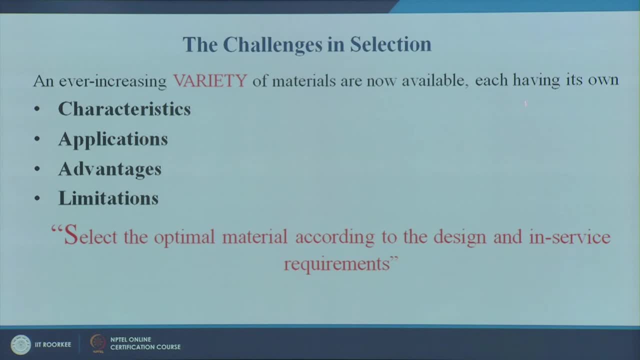 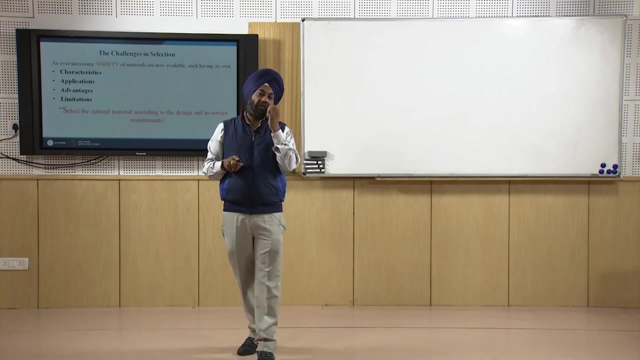 So that is the variety. But each material will have its characteristics, It will have its application areas, It will have its own advantages, limitations. Now we have to see that for our specific requirement, need, which material can satisfy that, So that we will select. 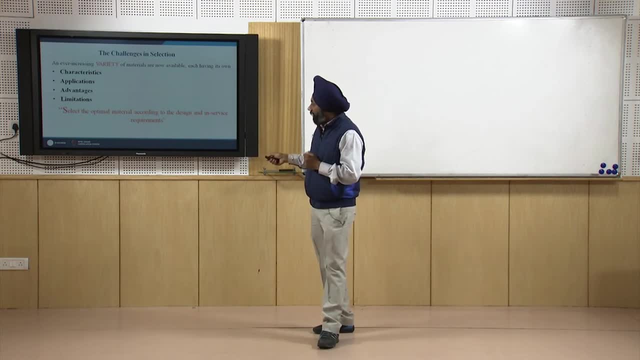 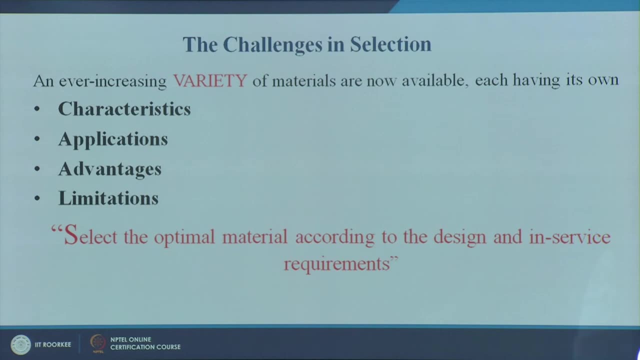 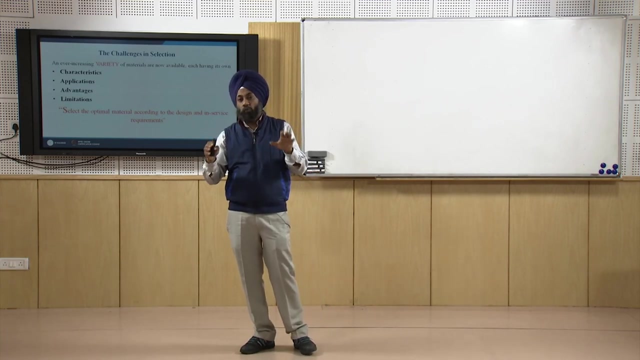 So we will select the optimal material According to the design and in-service requirements. As per the design of the product, we will choose that which material will satisfy our requirement. And second thing also, the in-service use means that when the product will be used, what type? 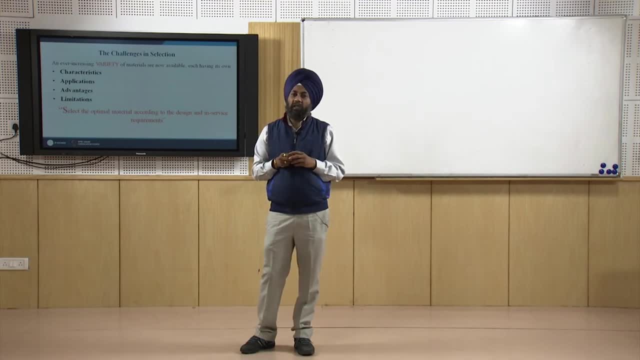 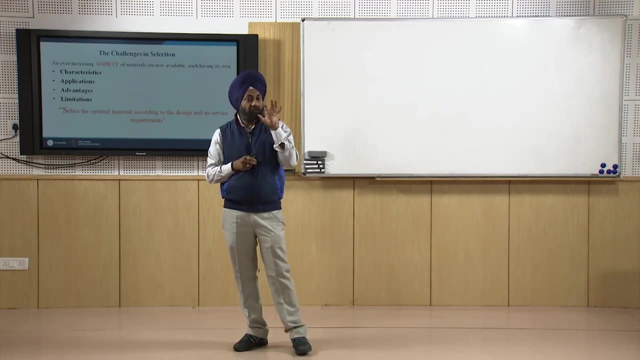 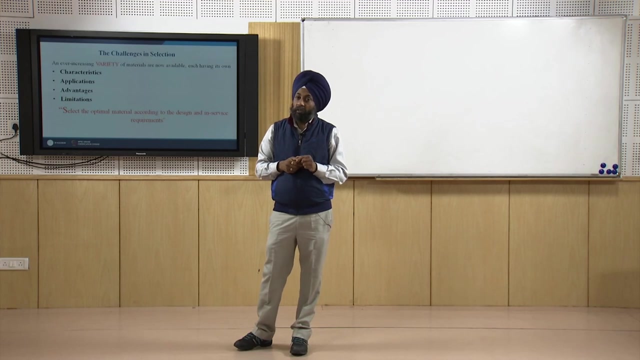 of conditions it will have to sustain, or what type of environment it has to sustain, or what type of loads that are going to act on that particular product. So the in-service requirement and the design, Both, Both will dictate the selection of the material for that particular product. 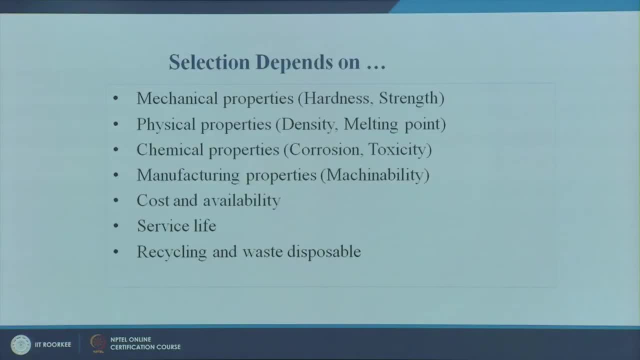 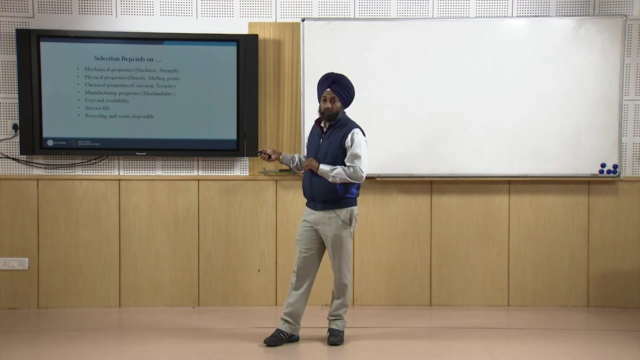 Now this selection will depend upon. It was very easy to say in the previous slide: select the optimal material. But how to select? We will select that based on the mechanical properties. We will see that. what are the mechanical properties that the product- sorry, not the product- that. 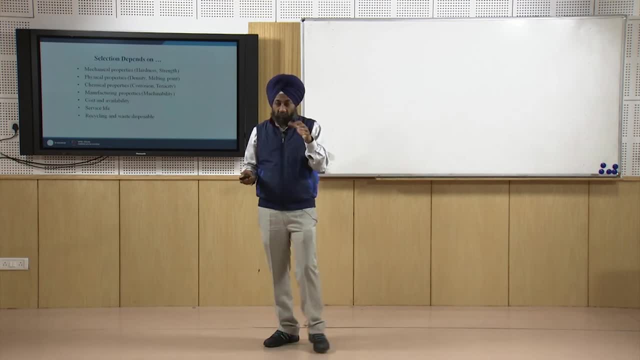 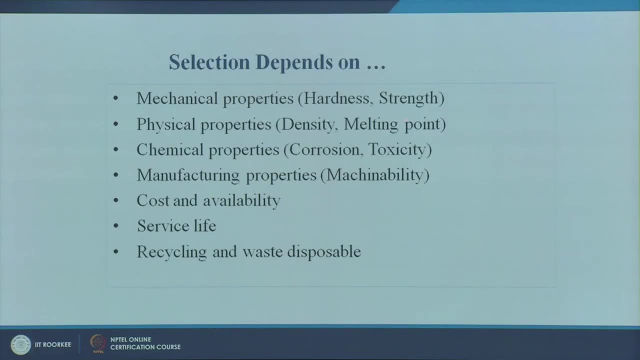 the material possesses, For example metal. Metal, We will see what is the hardness. what is the strength. For plastic also, we will see what is the hardness. what is the strength? Then the physical properties, such as density, melting point. Suppose we have application where the light weight is the prime design criteria. 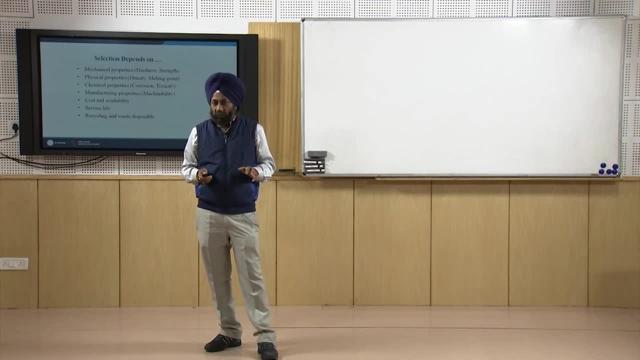 The product has to be light in weight. whatsoever may come and go Now for light weight product. what is the physical, we can say, property that we would like to ensure? We would like to see the density of the material that we are choosing for that particular product. 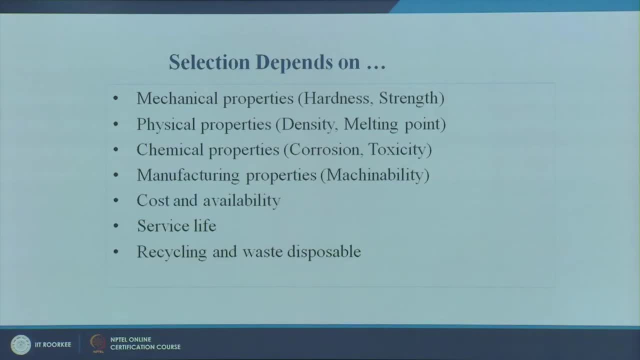 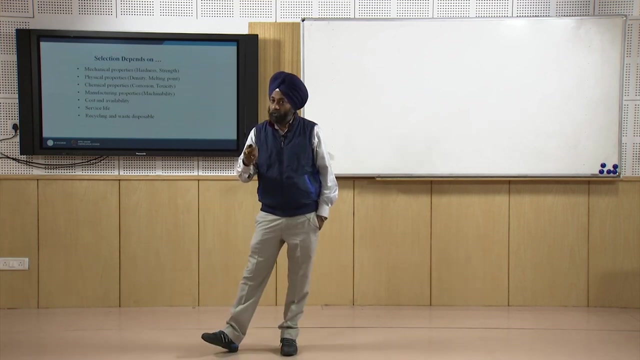 So your physical properties are equally important. So we will see the mechanical properties, physical properties, similarly the chemical properties, such as corrosion and toxicity. Now, for example, we want to select a material for food packaging requirement. So if the food has to be packaged in that particular material, it has to be non-toxic. 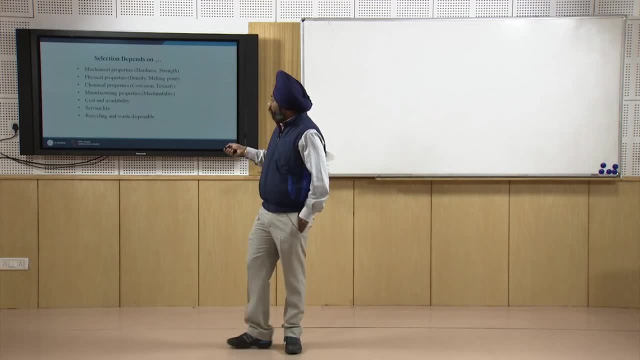 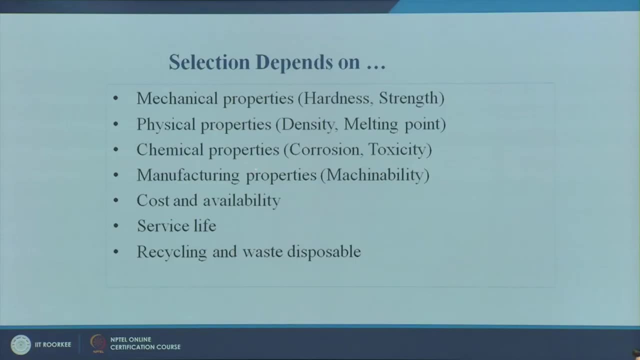 So that is a specific requirement for this application. So our selection of material for a particular product will depend upon the mechanical properties, physical properties, chemical properties, manufacturing properties, cost of the material, availability of the material, service life of the material, recycling and waste disposal. 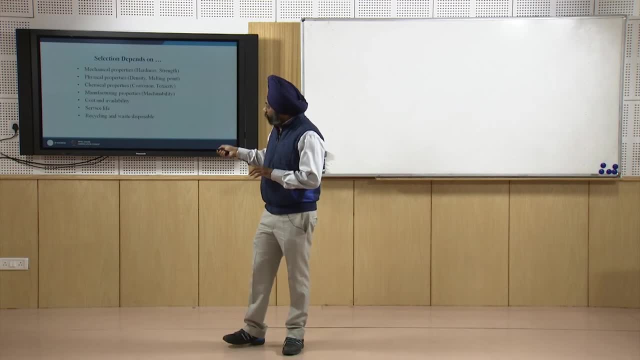 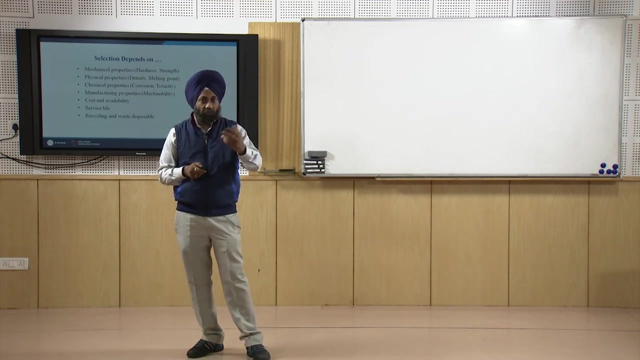 characteristics of the material. Now, each one of these points can be explained in a very, very exhaustive manner. For example, the last point. The last point: Recycling and waste disposal. There is lot of focus these days on selection of materials which are biodegradable, which? 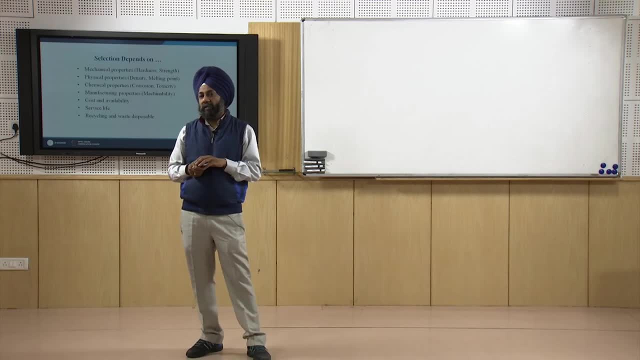 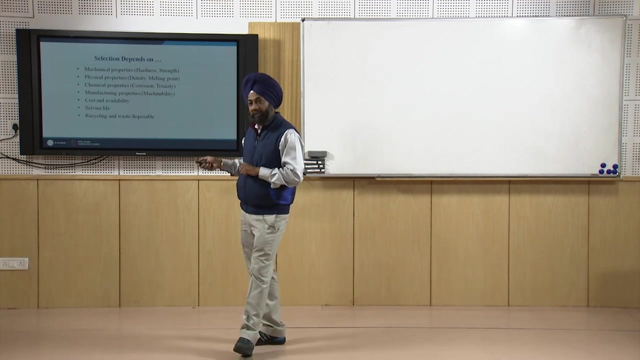 are recyclable. So most of the products that are made by non-biodegradable materials usually have very poor end of life characteristics. So these days, the trend is towards selection of biodegradable materials. Now, selection of material is equally important. Now what I expect. 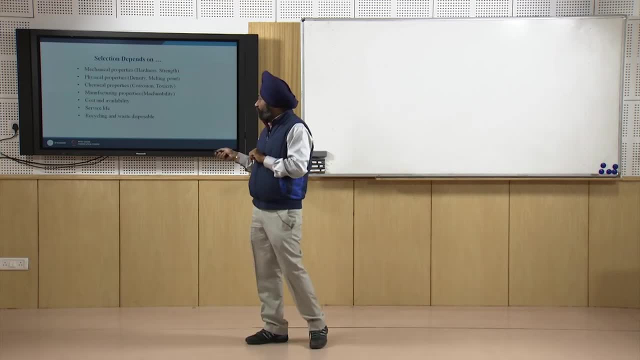 What I expect from all of you is that you can try to understand that where the plastics fit in in all these requirements. Because once you make a product using a polymer, you have to justify the cost, you have to justify the manufacturing properties, you have to justify the mechanical and the physical. 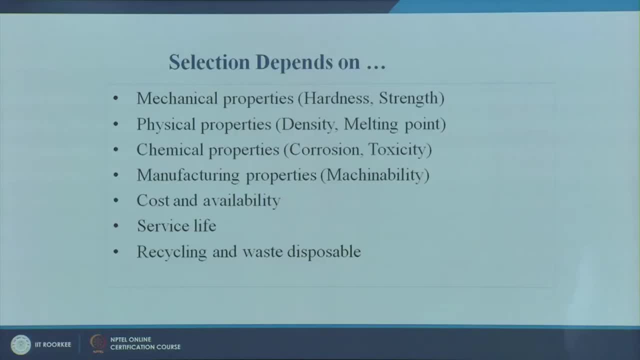 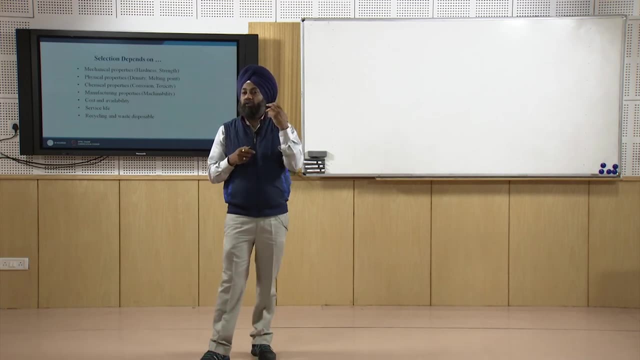 properties. Now our target is to study about the polymers and the polymer based composites. So once you propose, you postulate, You say Okay, That for this particular application a polymer based product should be used or, to simplify, that a plastic product should be used. 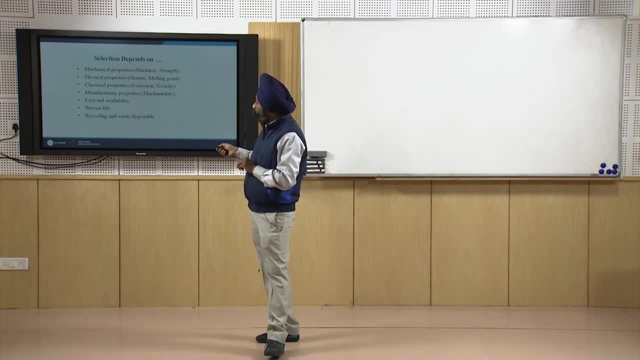 Now, once you say that you have to justify the use of plastic based on all these characteristics, and you have to compare based on all these characteristics, comparison with the other materials which can be used for making that particular product. So, once you think of, Think of polymer, 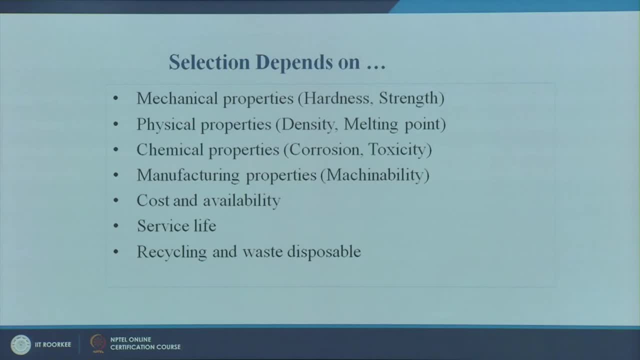 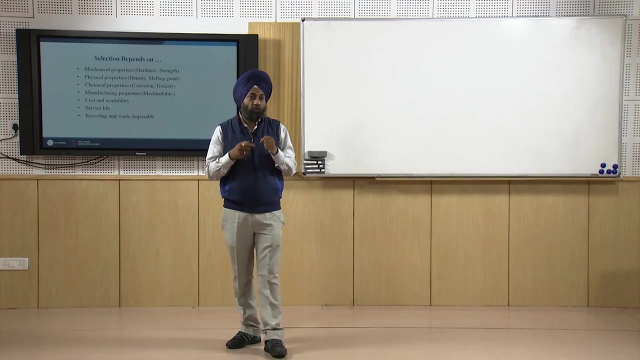 You have to think of polymer in all these context So that you are able to develop a product with that polymer. Because whatever we study, we study it for business, we study it for maybe application, and application will only come once you are able to displace some application with a new. 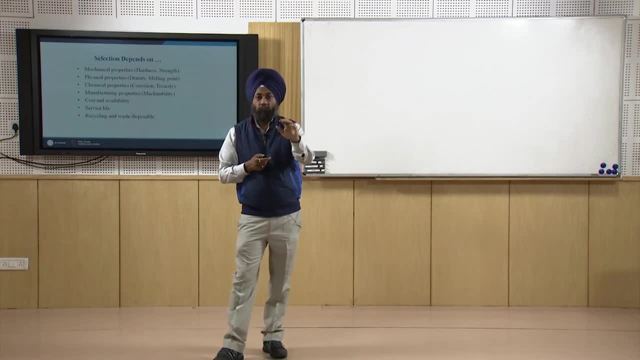 material. For example, a product is being made from a metal. Now you say that the same material is being made from a metal. Now you say that the same material is being made from a metal. Now you say that the same characteristics, same things, same in service requirements. 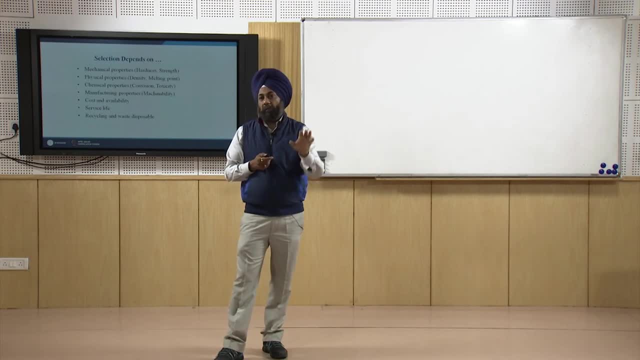 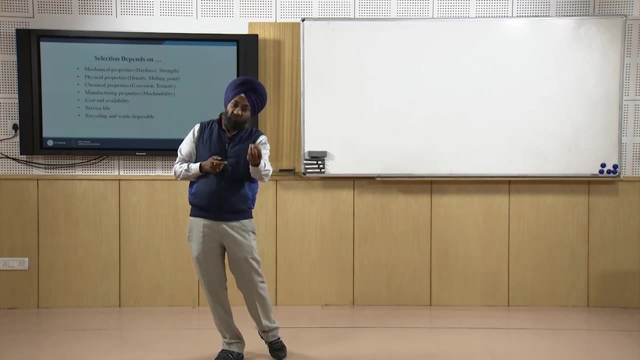 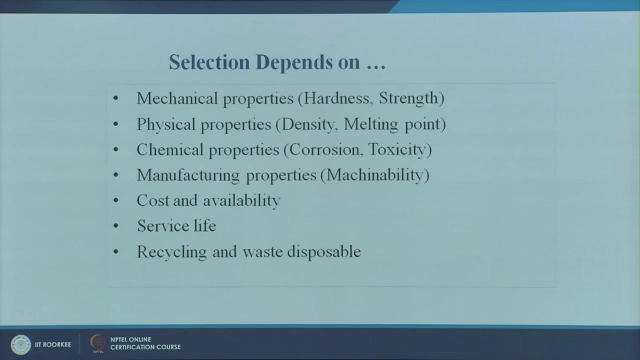 can be met if you replace this metallic product by this plastic product or a polymer product. What is the advantage? May be, density is less, So the weight will reduce, So that justification, comparison is only possible if you have this list in your mind. that where 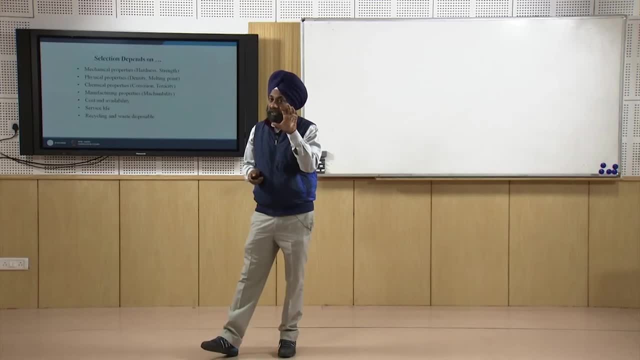 which material can be applicable. So your selection of polymer, Okay. So the manufacturing material will depend upon these characteristics, or this justification that you need to develop for proposing the use of polymers. Now, once that is done, we need to understand the types of manufacturing processes. 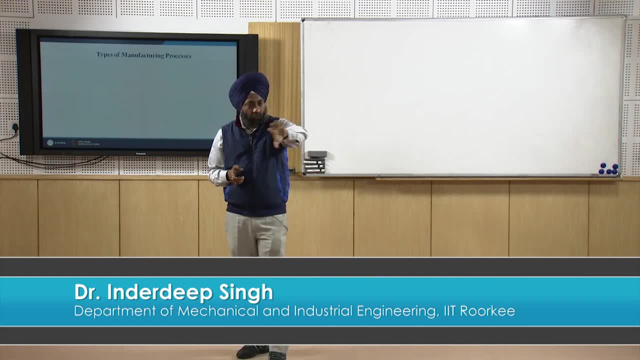 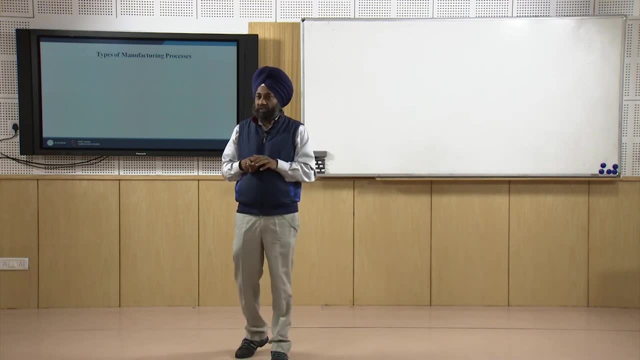 Now, once we have decided that a particular product is going to be changed, it is currently being made by wood, So wood is an important material. It requires cutting of trees, So we are going to replace that. Why a plastic material? So we make a justification based on the points which were highlighted in the previous slide. 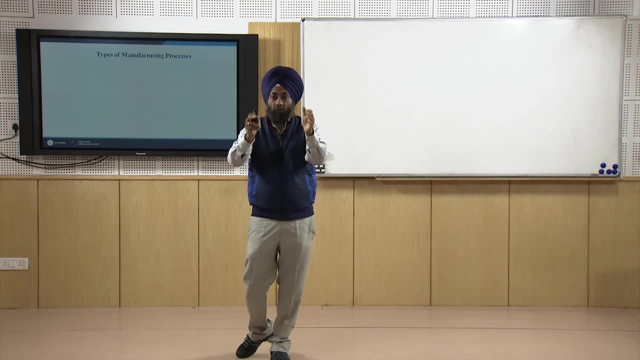 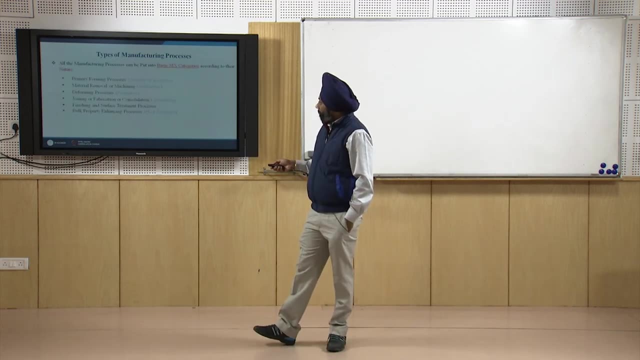 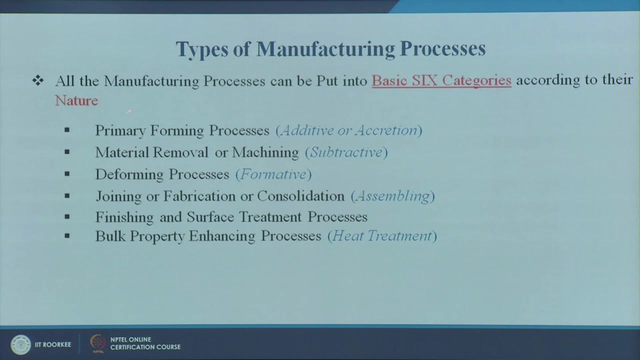 Now we have to understand that. what are the various type of manufacturing processes that are used for processing the engineering materials? There are broadly six categories. There can be primary forming processes, material removal processes, deforming processes, joining or fabrication processes, finishing and surface treatment processes and bulk property enhancing. 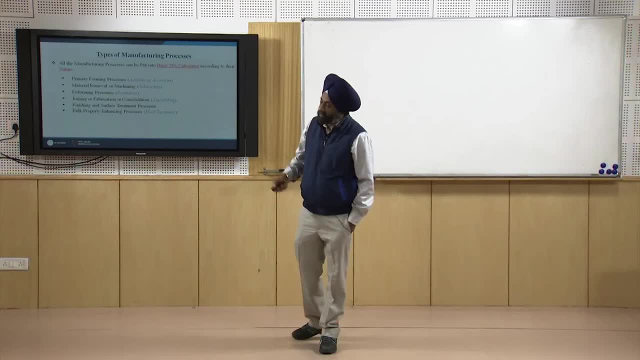 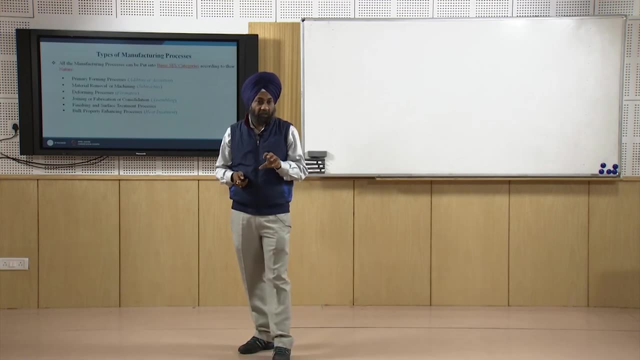 processes. Now for specifically polymers. I must highlight: primary forming processes are very, very important Now. primary forming processes are where we give a shape to the product: Your compression, molding, injection, molding, extrusion, thermo forming- all these processes, rotational molding- all these processes will fall under the primary forming process. 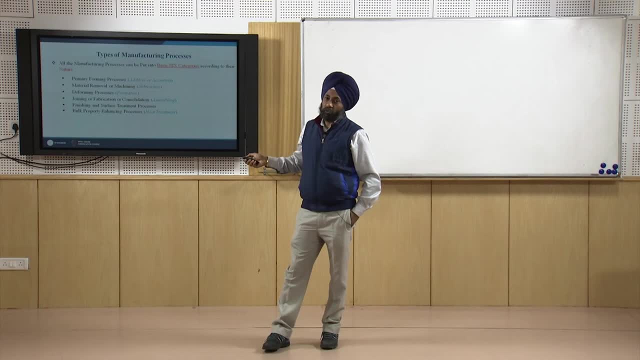 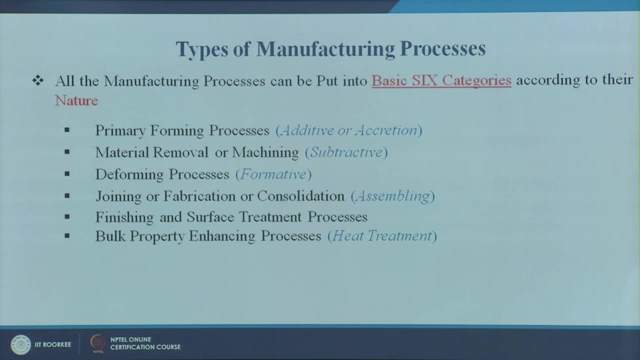 Okay, Okay, So these are the primary forming processes. So next is the material removal or machining processes. Sometimes you need to make a hole in a polymer plate or in a plastic plate. Sometime you may be required to cut a screws inside the polymer or may be threads inside. 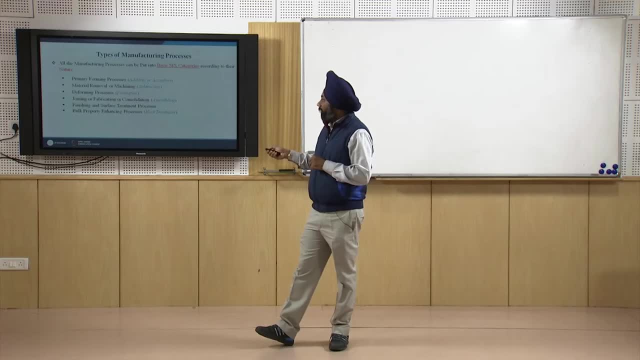 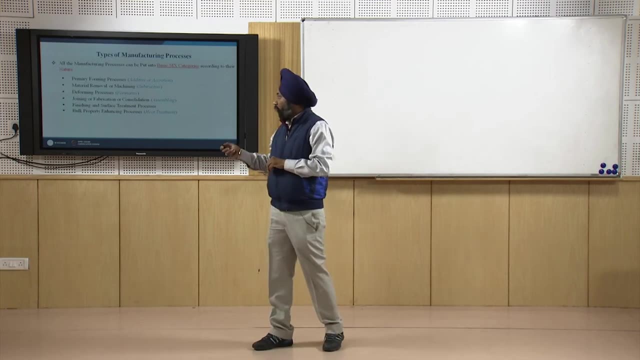 the polymer plate. So that will fall under the material removal or machining processes. Sometime you may need to do the edge trimming in order to fix the two parts together. So all that will fall under the material removal or machining processes. Okay, First are the primary forming that I have examples I have already given. 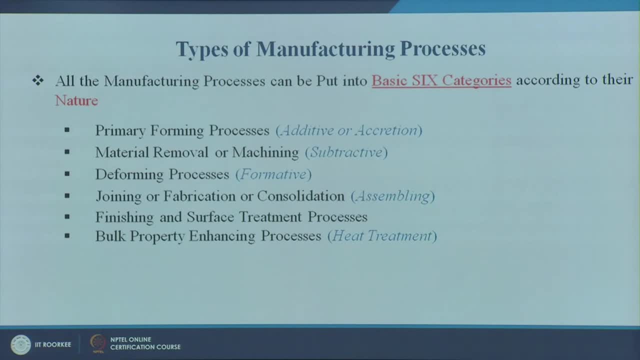 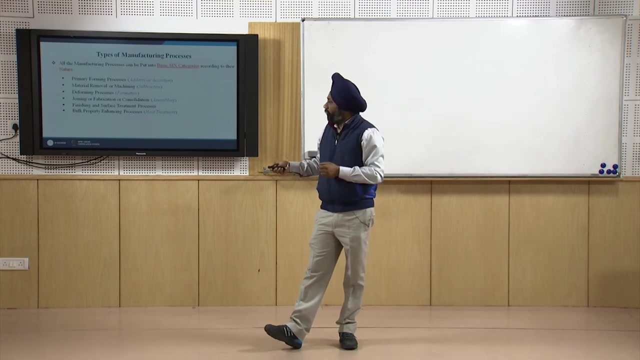 Deforming process is not very common in case of plastics because you mold the things in the primary forming stage. only You mold, you melt the plastic and give it a desired shape that we consider in the primary forming processes. But yes, sometimes we will make long tubes of polymers or plastics that we can say may. 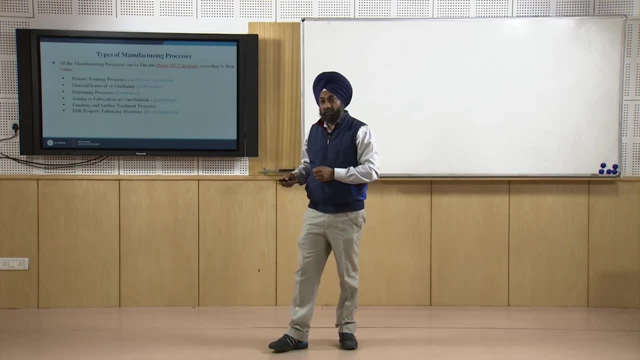 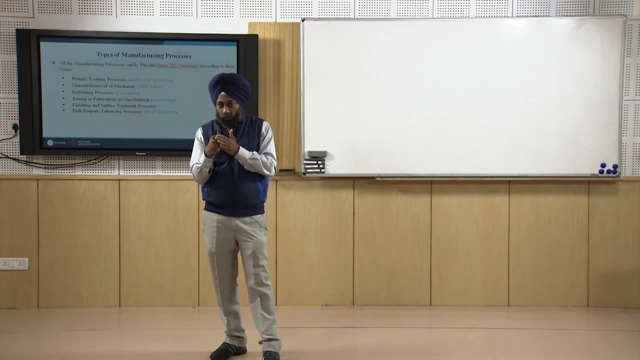 fall under the deforming, Then joining or forming, Then joining or fabrication. it is very difficult to join the polymer parts together. Difficult, I am saying because if you permanently you have to join, you need to do the adhesive joining, which is also a challenging task. 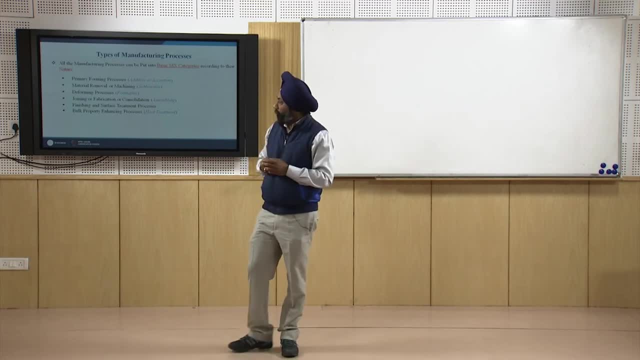 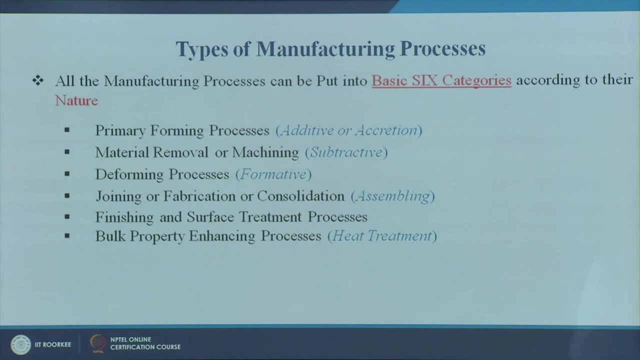 So we will see the joining behaviour of the polymers and polymer composites. But the joining can be adhesive joining, it can be mechanical, fastening. So those are the processes specifically for polymers. and then finishing and surface treatment, processing. So finishing and surface treatment in terms of plastics can be some specific coating on. 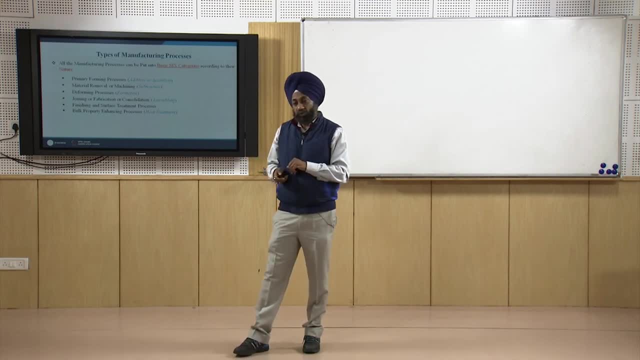 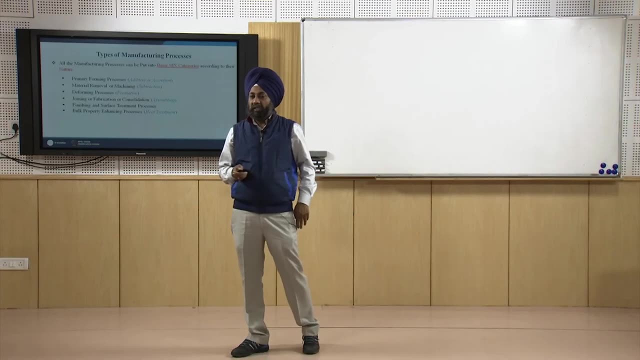 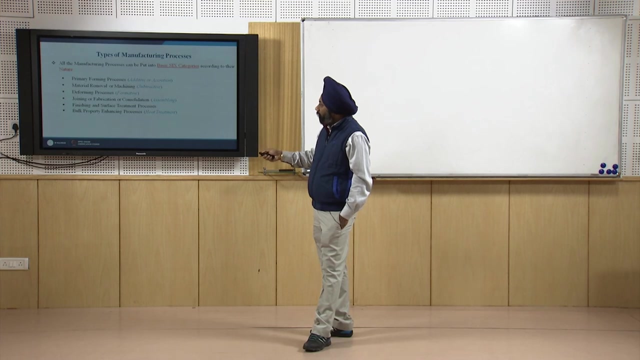 the surface that can fall under the surface treatment process. And finally, the bulk property enhancing processes such as heat treatment, which is very, very uncommon in case of polymers and polymer composites. So broadly, these 5 processes- primary forming, material removal, deforming, joining, finishing, 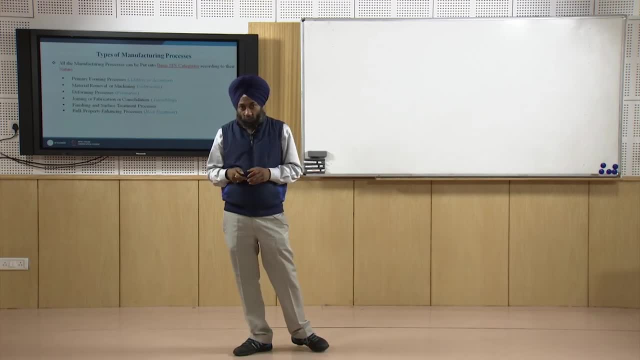 these are the processes which can be done on polymers and polymer composites. Okay, And if you see, all these processes can also be done. not only can also be done, but they are usually done for metals also. If you see metals, you can see the processes. 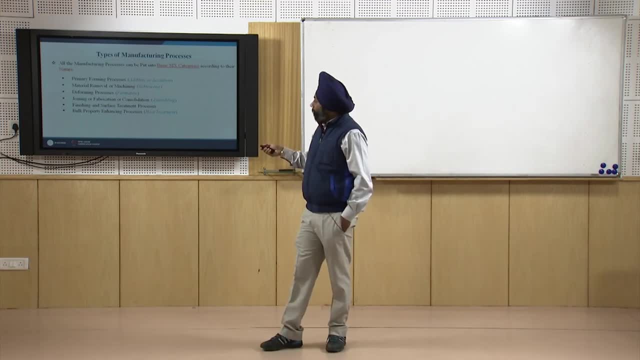 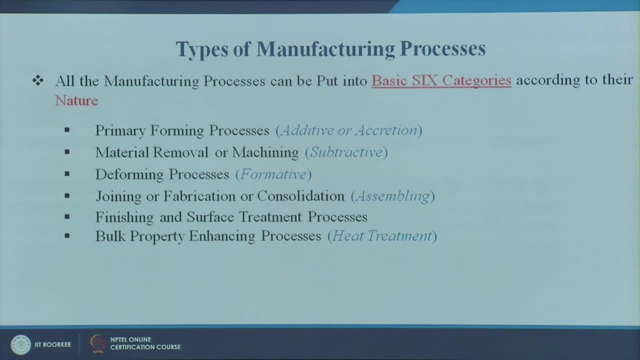 In primary forming. example can be casting, material removal, turning, drilling, milling. all processes will fall under the material removal. Deforming- it can be your tube drawing, it can be wire drawing, it can be extrusion, it can be forging. 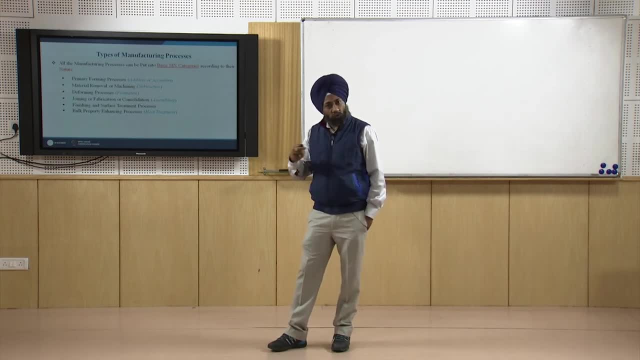 So you have processes like deforming. Joining may be most common. welding is one of the most important process for joining. Finishing grinding is one process which is used for finishing And bulk property enhancing, such as heat treatment. there are number of annealing and then there 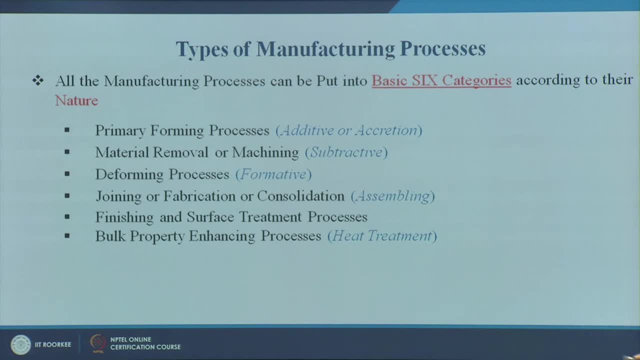 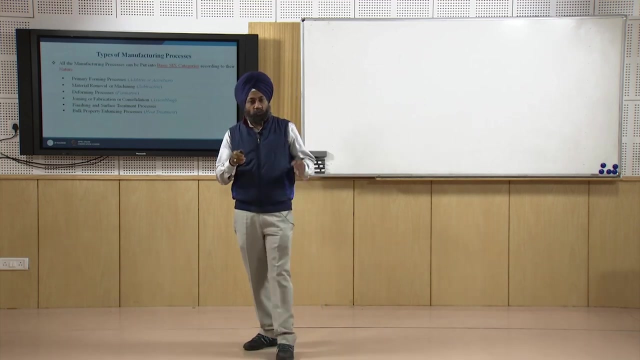 can be hardening or sometimes it can be austempering, martempering number of processes which are falling under heat treatment category. So if you see, for metals all these processes are well developed and this classification holds good For metals. but as soon as you go to plastics you have to think that which process will? 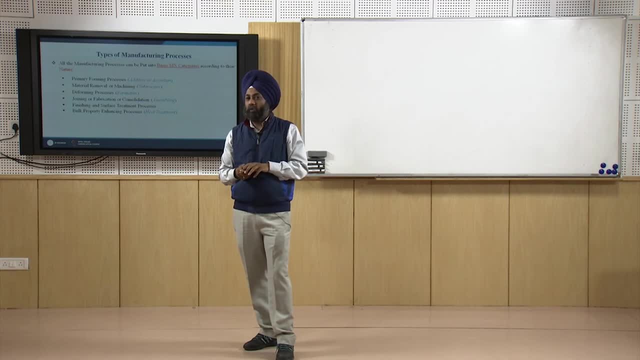 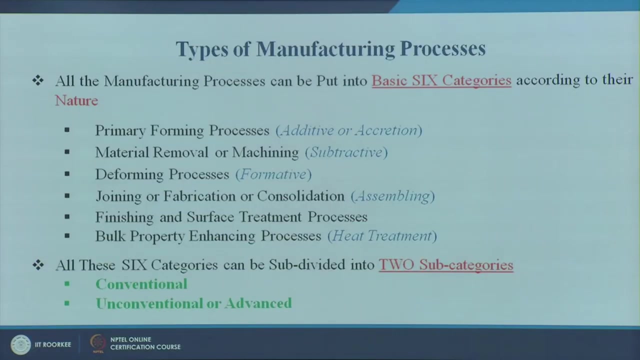 fall under the primary forming, which process will fall under the joining. So most of the processes are not very well developed for polymers but are very well developed for metals. that we will try to understand with the help of a slide. So further, these processes can be further categorized into two parts. 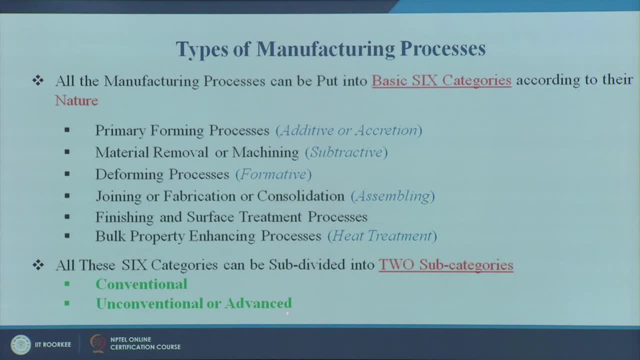 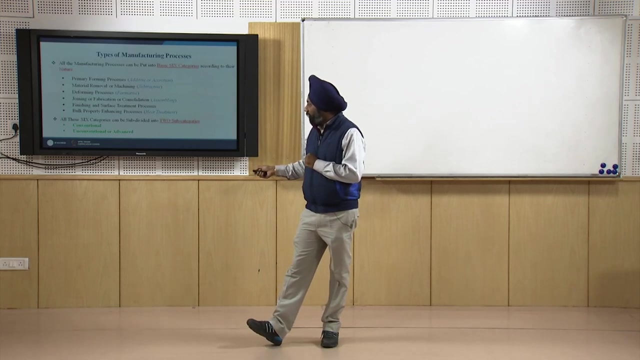 They can be either conventional processes or they can be unconventional or advanced processes. We will see mostly the conventional processes, but towards the end, when we go to the material removal of polymers and polymer composites, we will see some advanced and unconventional processes also that are specifically dedicated towards the polymers and the polymer based. 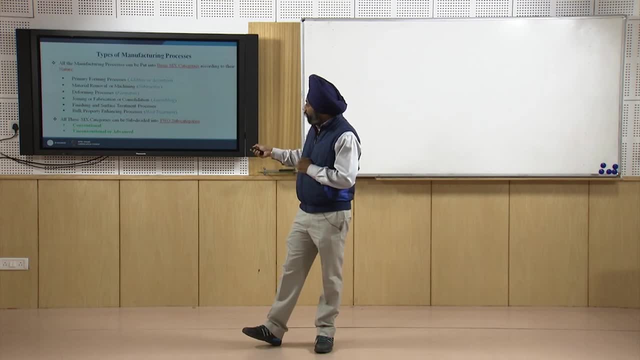 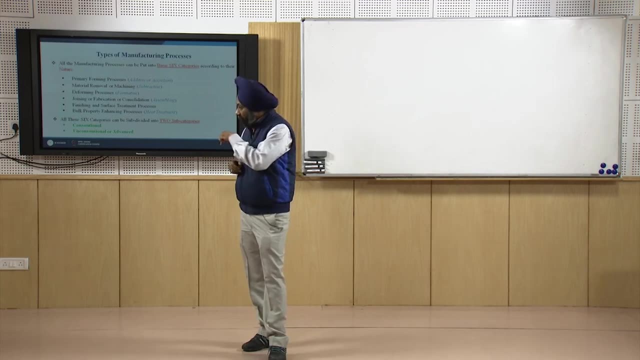 composites. So this is a classification of manufacturing processes. I have tried to bring two things into picture. One is classification specifically for polymers And the second is classification specifically for metals. So the similar classification holds good for polymers also and for metals also. 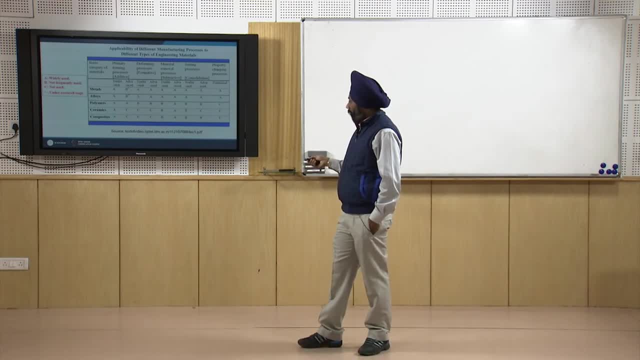 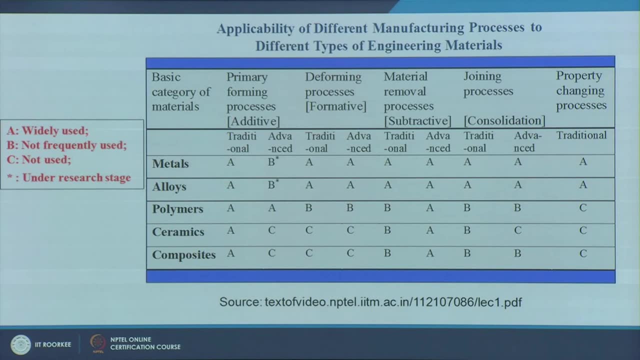 Now, this is a important slide taken from a particular source available in the book also. So here you can see A means widely used, B means not frequently used and C means not used. I will just ask you regarding polymers, you can see A A, B, B, B, A B, So only property. 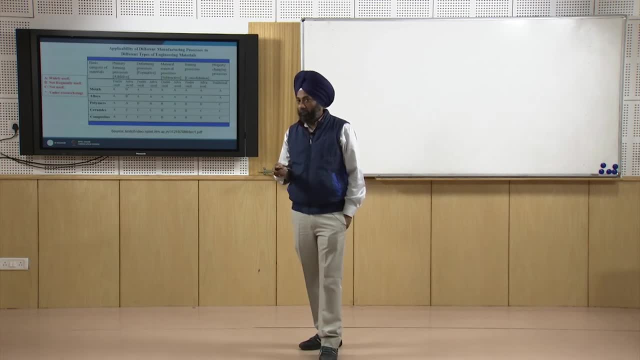 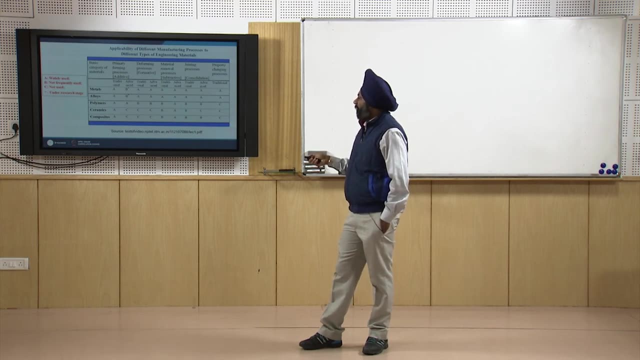 changing processes, which I have already told. the heat treatment process is not very common. for the polymers C rest all A and B, which means widely used processes and not frequently used processes. So if you see polymers primary forming widely used both in the traditional and the advanced 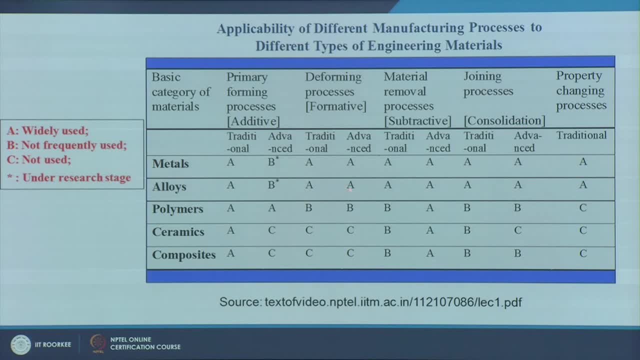 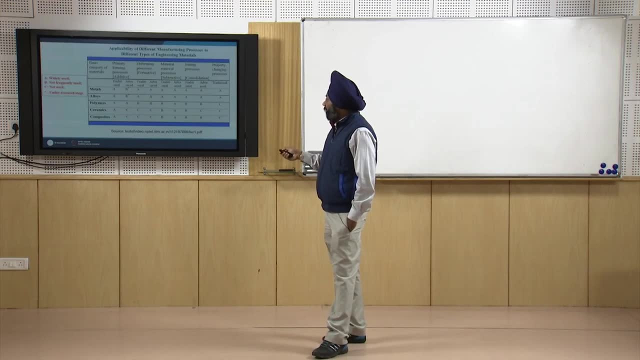 method. Deformative processes may be not widely used, as I have also given example that deformative process is not very common. Material removal processes for polymers: yes, advanced processes are there, which I have also told that for this we will go to the advanced processing of polymers and then joining. 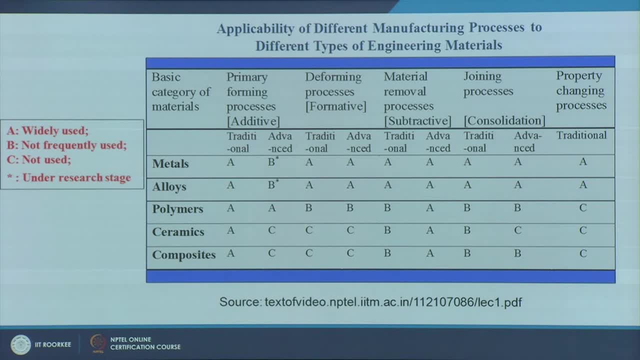 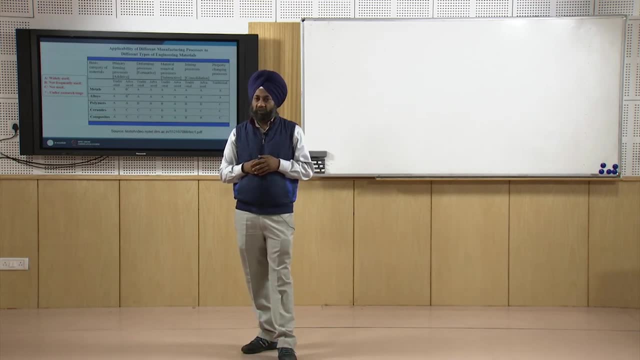 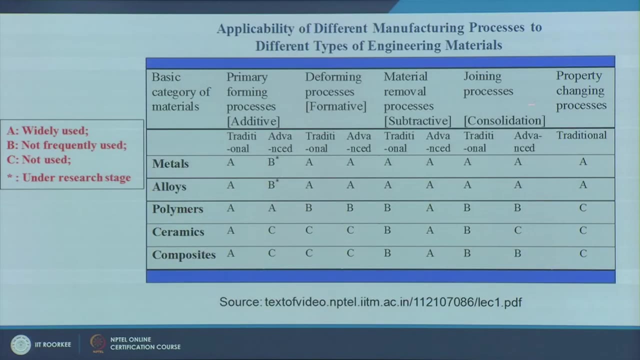 processes B and B not widely used because, I have already told, there is challenge when you even use the adhesive for joining the two polymer parts together or two plastic parts together. So this slide gives you an overview of the processes that are dedicated for processing of polymers. 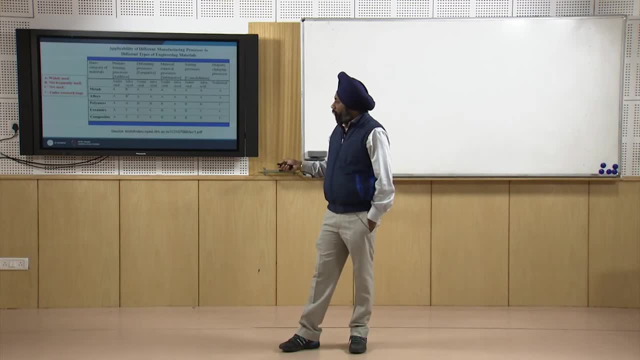 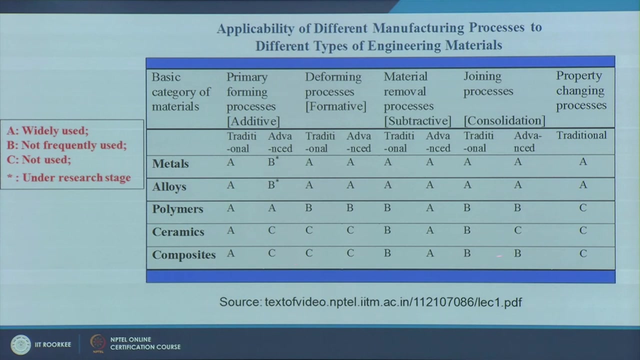 Now, one more thing I want all of you to see is the composites, because our title is polymer composites, also processing of polymer composites. So you see, for composites C, C, C that is not used, C Number of Cs. are there number? 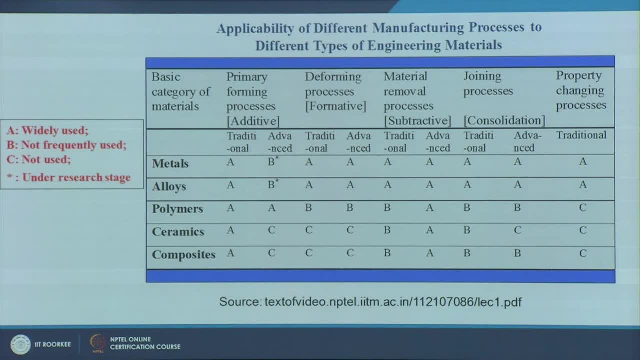 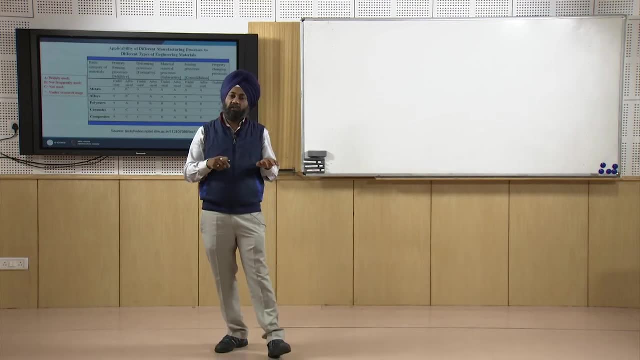 of Bs are there, so A is only 1 and 2. So only two processes we can say are widely used for processing of polymer composites. rest, all processes are either not used or are under the research stage. Therefore the topic becomes even more important as engineers that we should know that. what 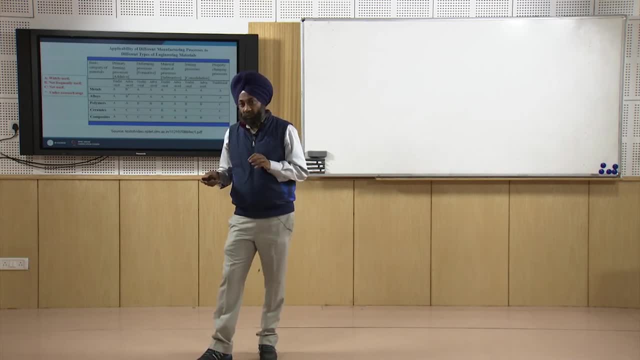 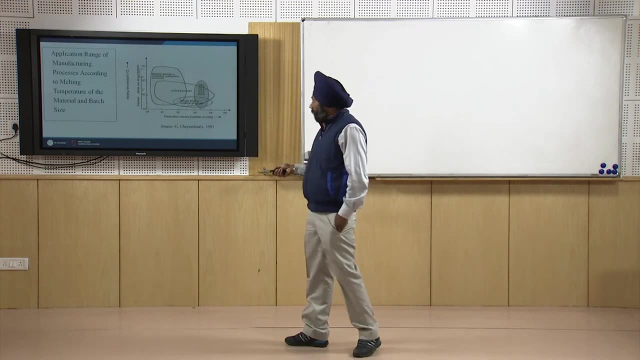 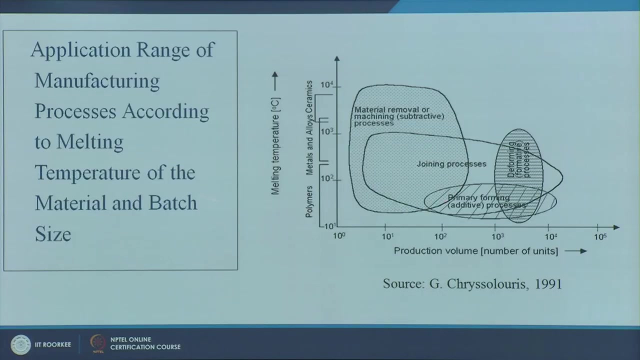 are the processes which are widely used for polymers, processes that are being used for polymer based composites. Now this is another taken from this source in 1991. this diagram was may be published. Application: range of manufacturing processes according to melting temperature of the material. 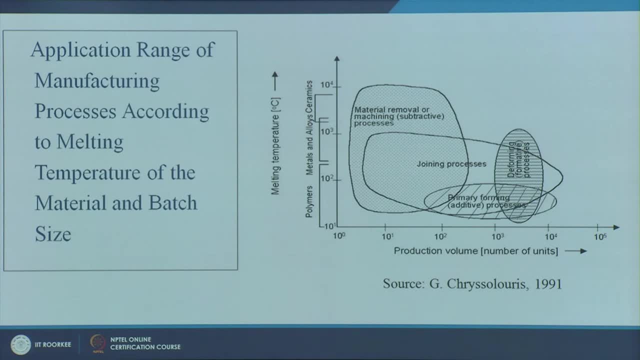 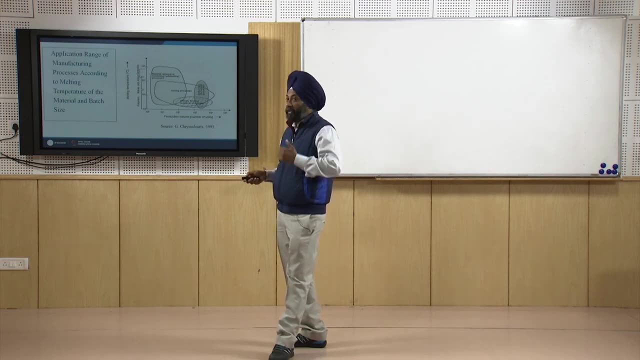 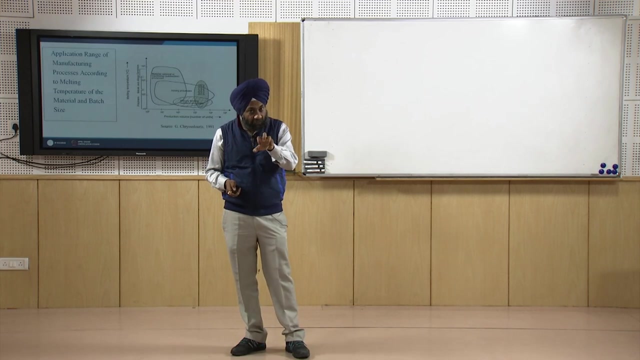 and the batch size. So when we have to select the material, we have to see that how it will be processed and, for processing point of view, we have to see that which process would be suitable for making that product. Now, when we have to select a manufacturing process, we will see such type of information. 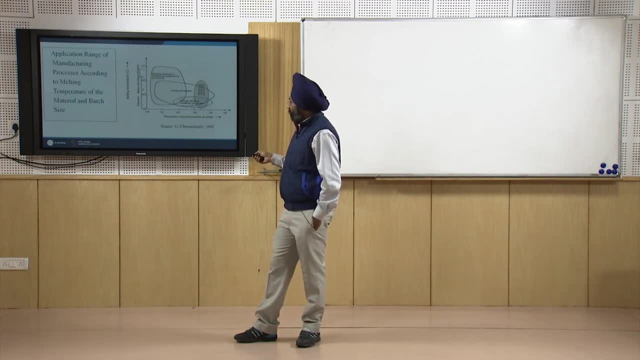 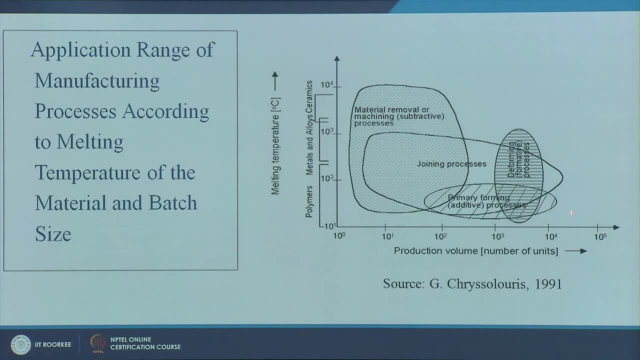 is available. If you see, the production volume is less. material removal processes are most commonly used And when the production volume is very large, the deformative type of processes are majorly used. So, from production volume point of view, if we have to- which means if we have to make- 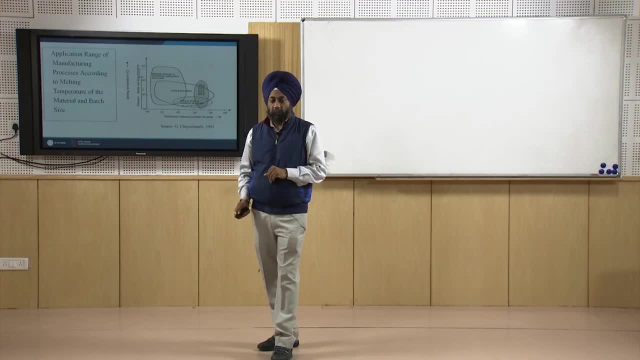 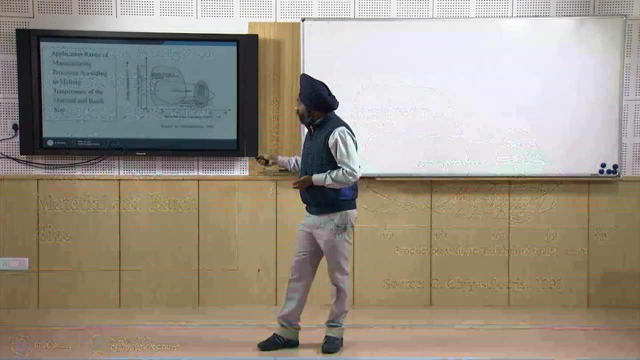 smaller number of products, go for the machining route. If you have to make a larger number of products, go for the deformation route. And, from the melting temperature point of view, which is very, very, very, very common in case of polymers and polymer based composites, 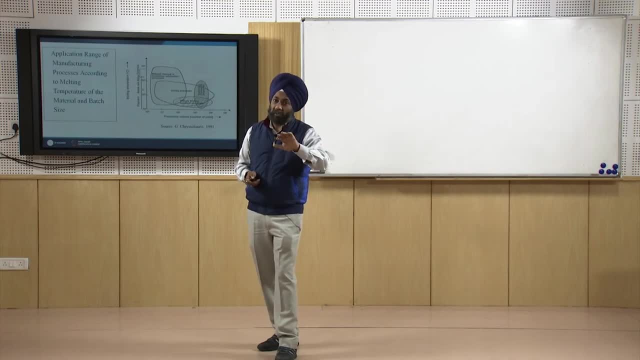 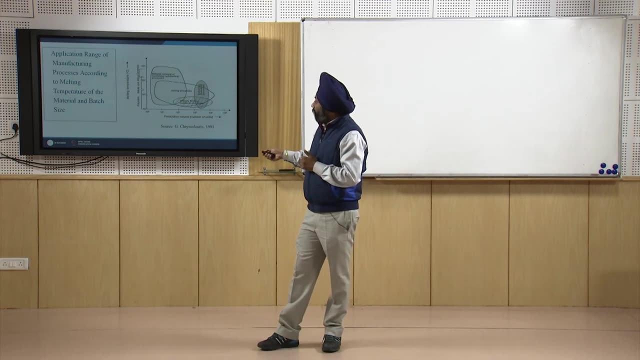 The volume may be, from industrial engineering point of view, important, but from technical engineering point of view, The melting point of view, the melting point is very, very important. So you see that when the melting point is less, the polymers are falling under this category. 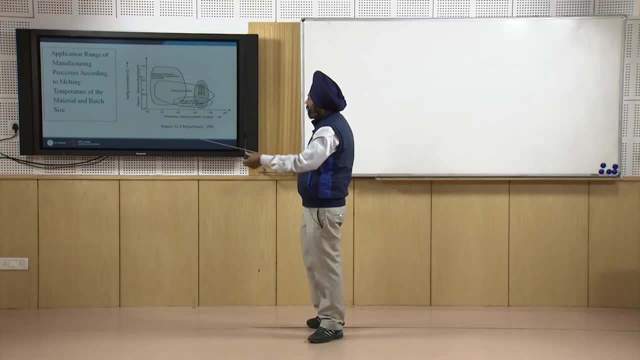 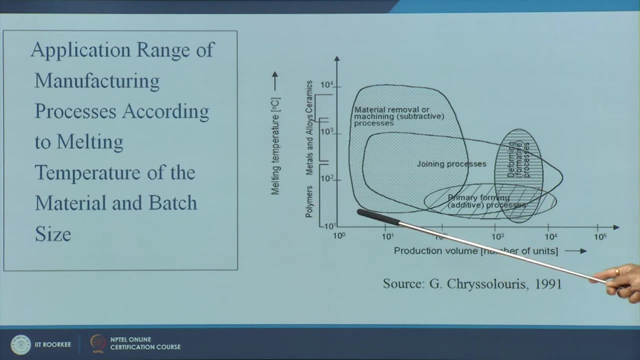 Again, I would like to highlight, because this is an important slide. you can see the polymers you can see are falling here. So the temperature or the melting temperature for polymers is less. So you see, the primary forming processes are most common for the processing. 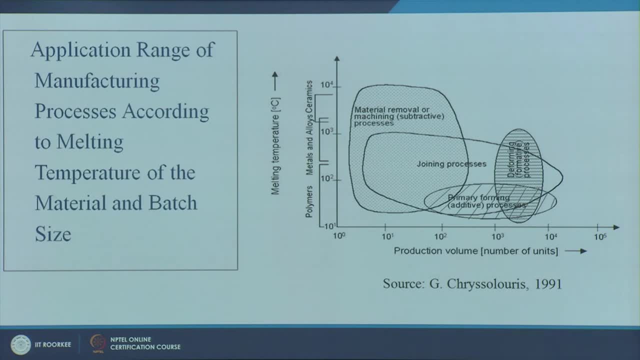 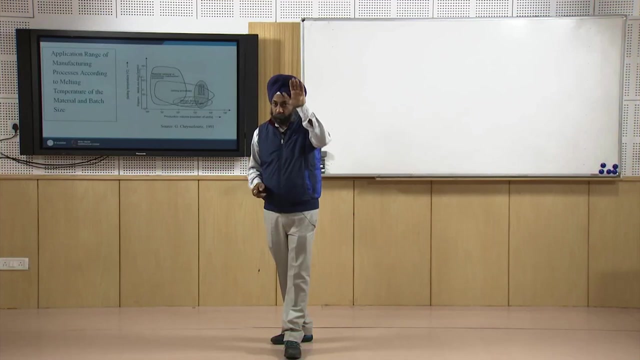 Of polymers. So we can conclude from this particular slide that the melting temperature for polymers is less and therefore the primary forming processes are most common for processing of polymers, And we will see the different primary forming processes that can be used for processing. 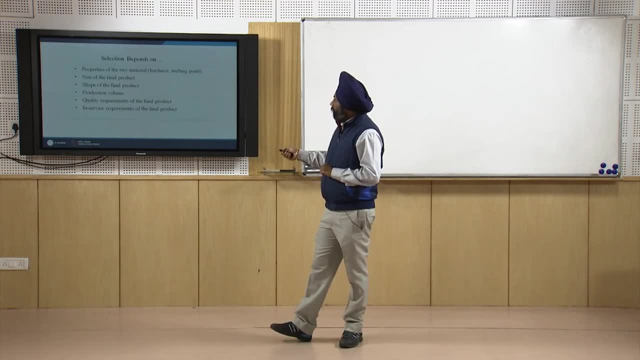 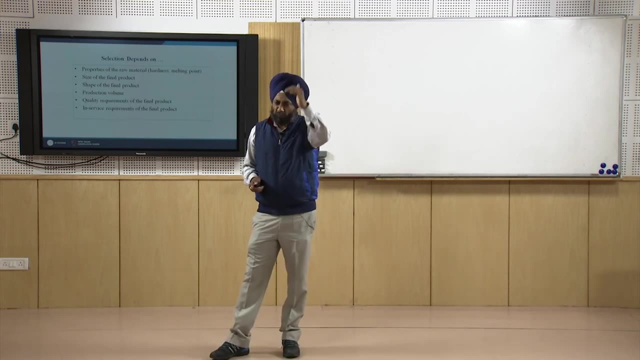 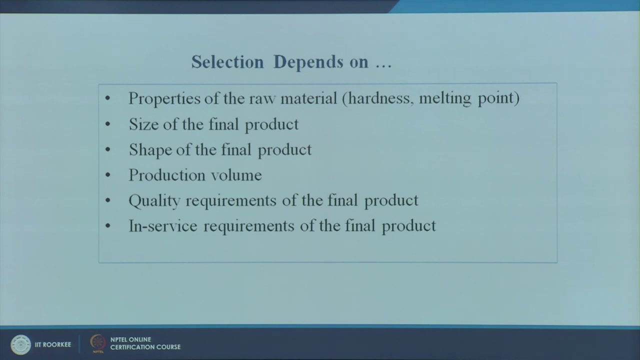 of polymers. Now the selection of the manufacturing process will depend upon. as we have seen, the selection of engineering material will depend upon so many parameters like mechanical properties, physical properties, chemical properties, manufacturing properties, cost and availability. Here we will see that the properties or the selection of a particular, we can say, process, 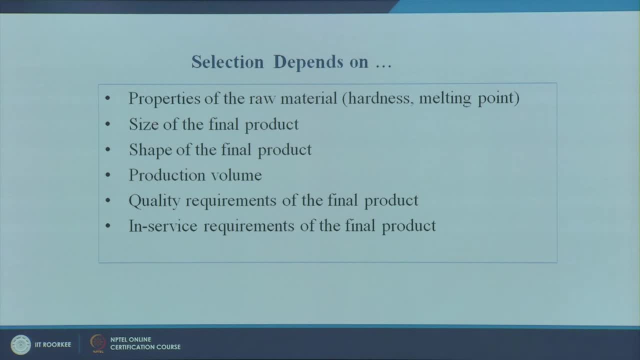 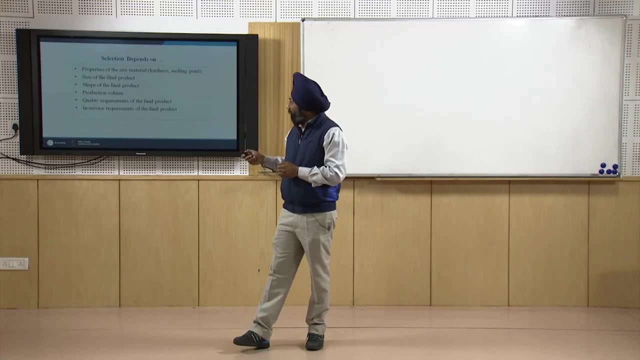 will depend upon the properties of the raw material, the size of the final product, because this is a smaller product. if I have to make a very big product, the process has to be different. It will depend upon the shape of the final product. if the shape is simple, you will select. 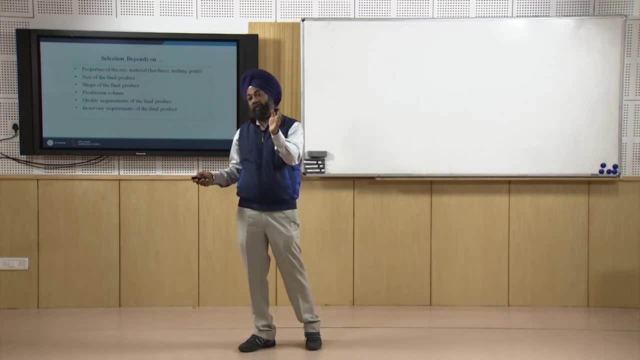 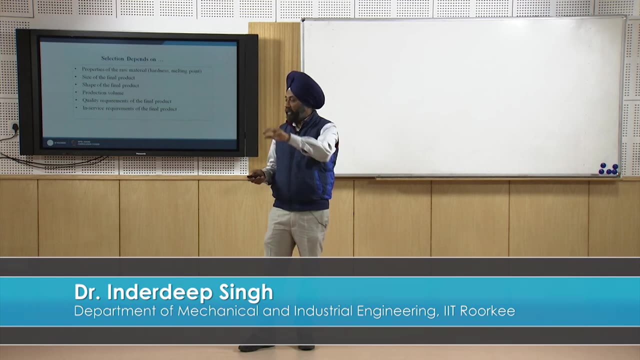 one process. if the shape is complicated, you will go for a different process. So for a small size, different process. large size, different process. simple shape- different process. complex shape, different process. Then the production volume: how many products you want to make? you want to make 100 products. 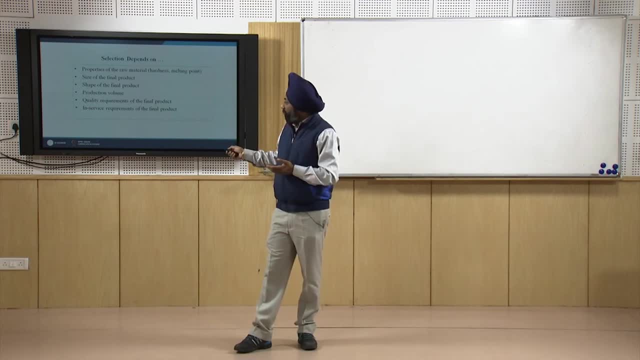 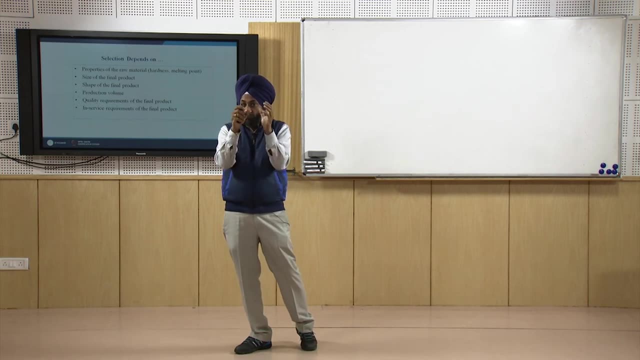 or you want to make 1 million products, So you will select the process accordingly. Then the quality requirements of the final product: what type of surface finish you require, what type of surface characteristics you require. that will dictate the selection of the manufacturing. 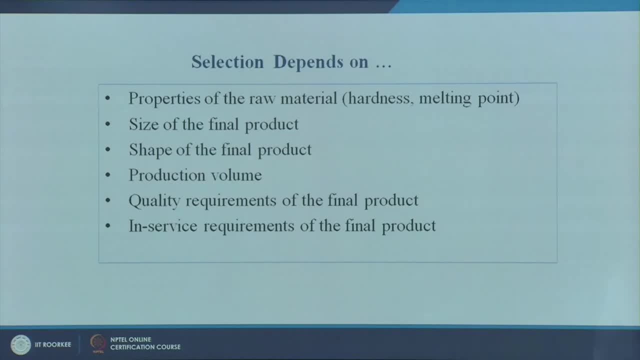 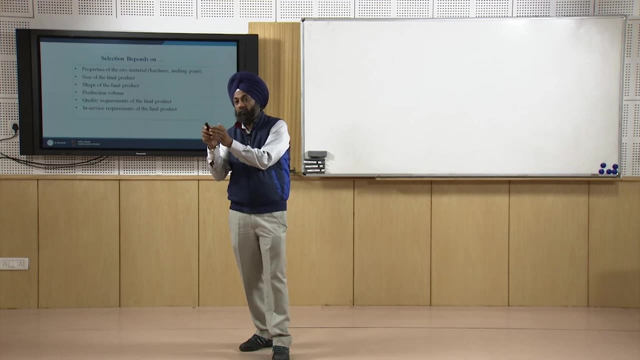 process. Also the in-service requirements of the final product, because the processing technique will also affect the properties of the material and the properties will further affect its behaviour once the product is put into service. So we will try to understand each one of these things, that which process.